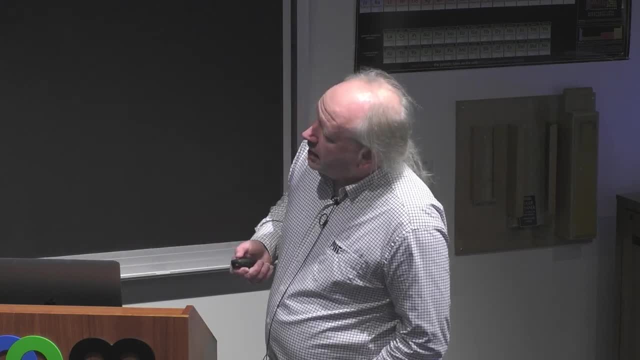 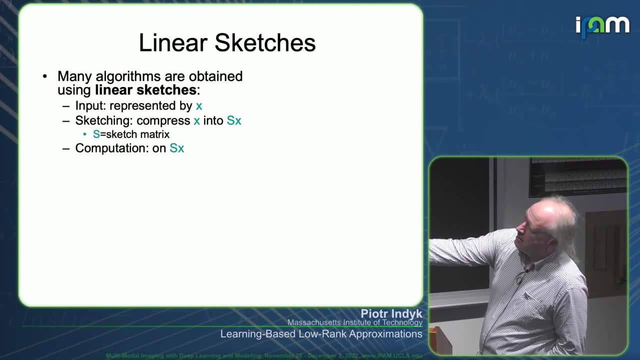 And there are also other names. No matter what the names are, the goal of this compression here is to reduce the dimension of the vector Right. So this is a. So this is a dimensionality reduction. step x is larger than S of x. 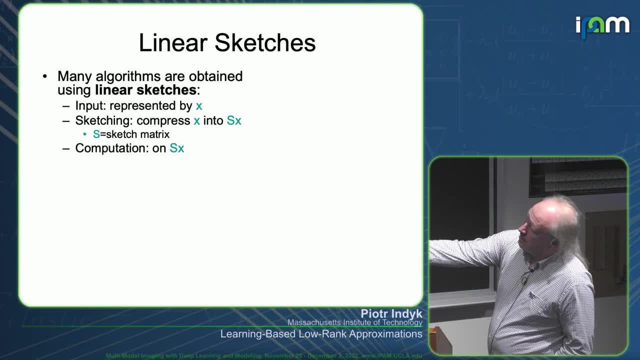 Okay, And once the algorithm performs this compression, then the rest of the computation is performed on the sketched version, as opposed to the original version. Okay, And, as you can imagine, the reason for doing it are numerous. You know for one, if S times x is shorter than x, then operating on the sketched version is a little bit faster. 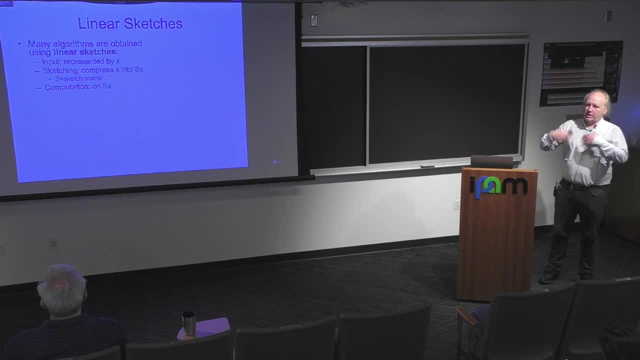 can be much more efficient, right, So you can save space time. you know, you can use it in various architectures that you couldn't use otherwise, and so on. All right, so what are the examples of this approach to algorithm design? You know, the prototypical example is a compressed sensing. 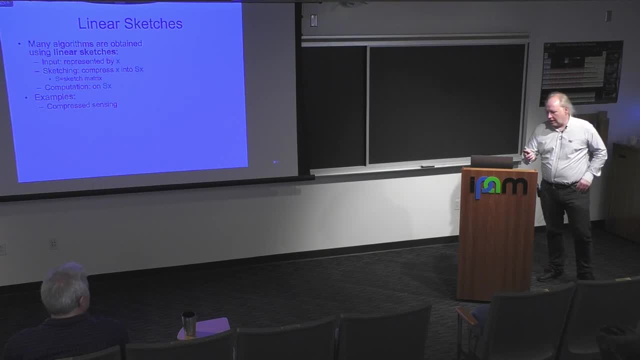 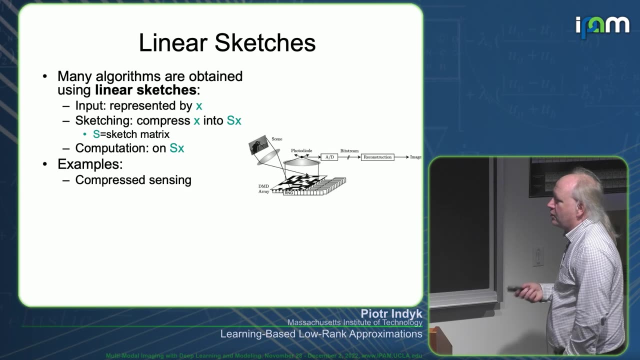 right, which I'm sure that most, if not all, of you have seen it before, right? So this is a classic picture of a single pixel camera developed in a Baranyuk and Kelly group at Rice University. All right, so you know. the essence of this camera is that, instead of you know, you have an. 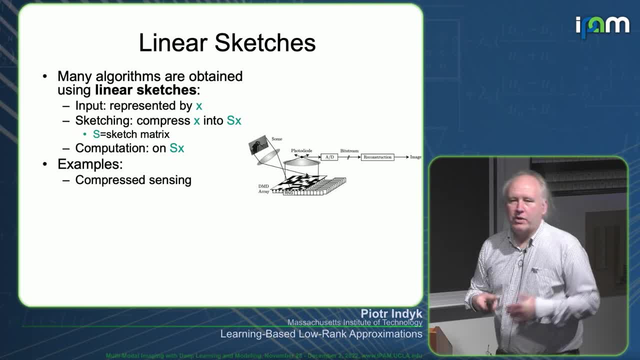 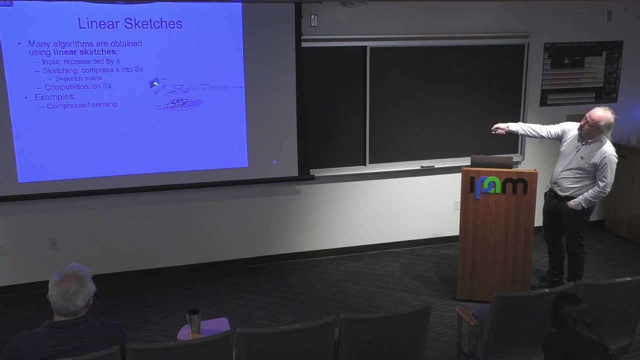 image, instead of sensing this image pixel by pixel, which would require either lots of sensors right, or a long time to scan, you know. instead, you, this device, you know, computes a projection of this virtual vector describing the image with, or computes a dot product of this image. right, with some. 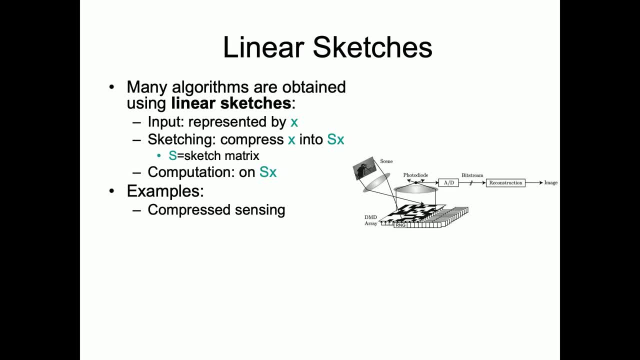 pattern, a pseudo-random pattern, and then this value of this dot product is being sensed by a single sensor. okay, So this makes it possible to acquire the image using, you know, in this particular case, only a single sensor, and if you do it several times, you're going to get several. 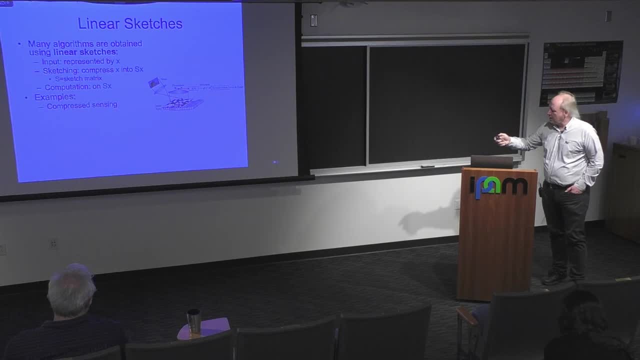 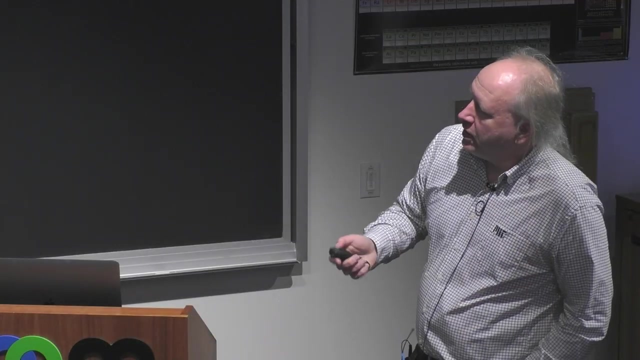 measurements of the image using those random vectors, and then you're going to get a single sensor And from this relatively few number of measurements, compressed sensing theory in practice shows you can recover X okay. So this is one perhaps the most well known example of you know this class of algorithms. 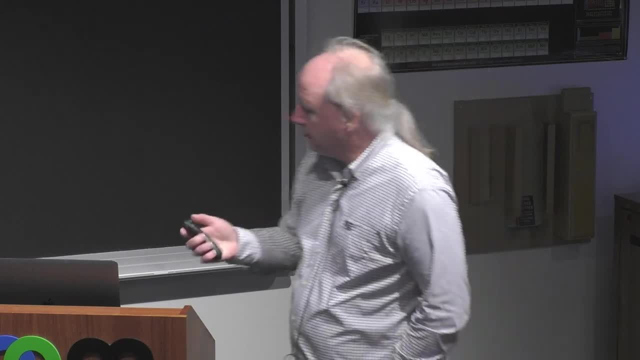 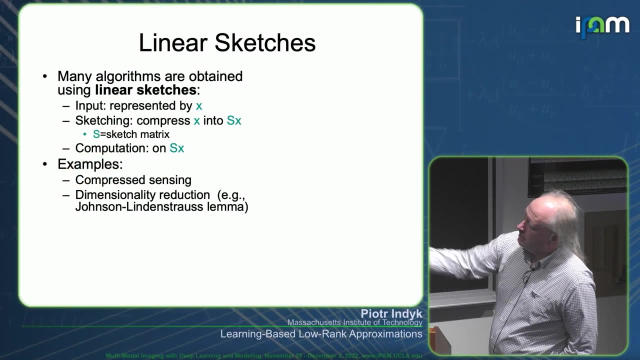 There are others. So in the project of compressed sensing, at least part of the theory is based on the random dimension reduction theorem due to Johnson-Liedershaus, which essentially says that if you have a bunch of points in a high dimensional space, you can hit them with a random matrix. S reduce. 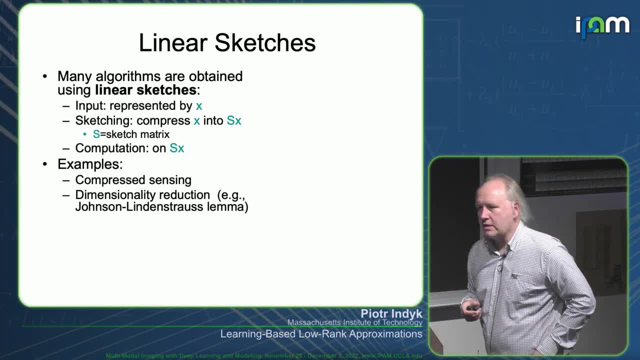 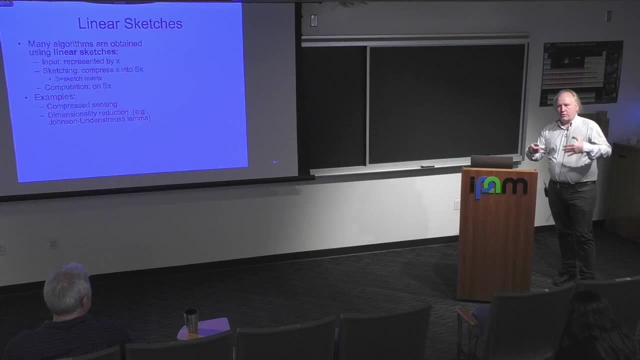 dimension while preserve the distance properties of this input, And compressed sensing is one application of aspects of compressed sensing are one application of dimension to reduction. there are others like, for example, nearest neighbor search or other algorithms which also use this method, And there are many other areas. right like I work a lot on streaming algorithms, the 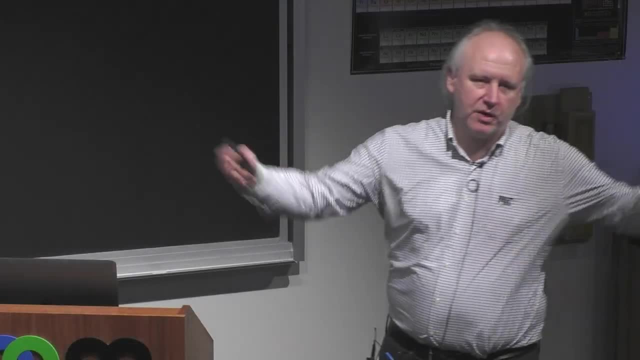 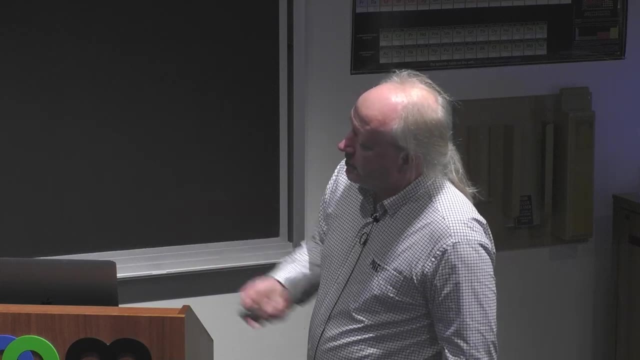 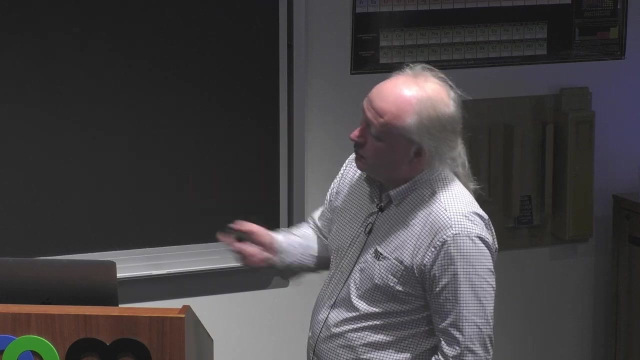 algorithms that use very little space, right, and the reason why they use very little space is because the whole input is compressed right, so that you don't have to store the whole input, And so on and so on. For today, we'll just we'll focus on one particular class of algorithms, which are 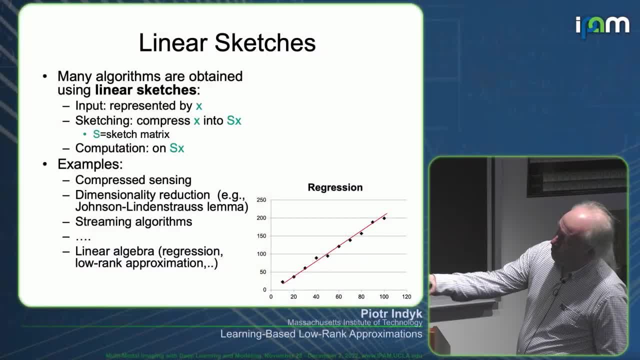 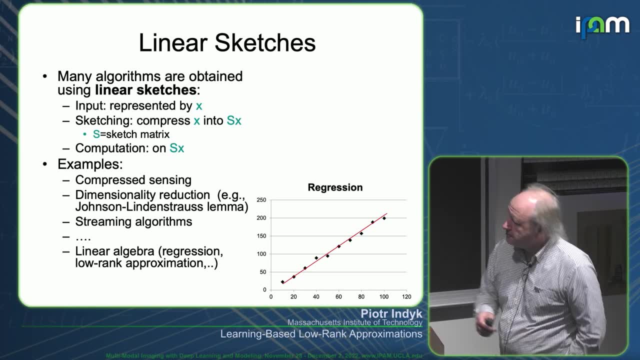 algorithms for linear algebra and in particular, for problems like regression and low rank approximation. So, as we'll see, over the last 15 years or so there have been lots of developments in fast approximate algorithms for these problems, and most of those algorithms use sketching. 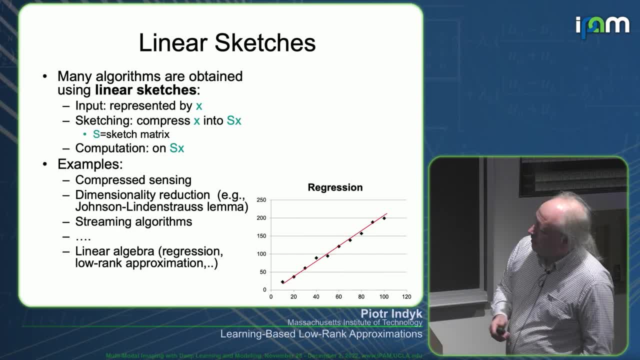 as a key component. okay, So in the rest of this talk I will give an overview of this experiment. This is a class of algorithms, and then I will describe. you know how we can use machine learning to improve upon this algorithm, in particular how to learn these matrices S. 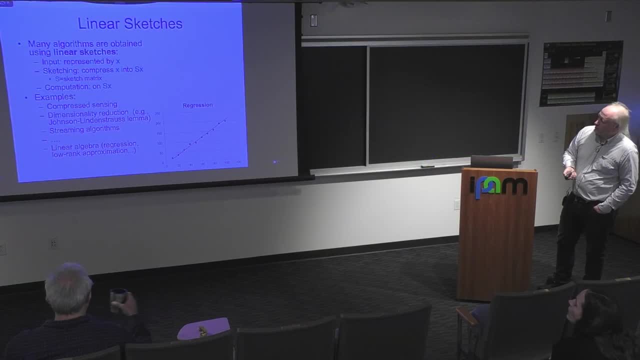 right to improve the performance of those methods, All right, all right. so I kind of said it already, but you know I'm just gonna repeat again. So in the rest of this application the matrix S is chosen at random. right, there are various. 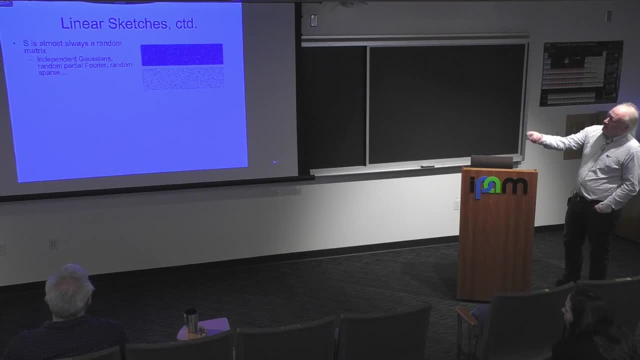 distributions to choose it from and they are not all equivalent. right, you could use independent Gaussians. you know random partial Fourier, random sparse- right. but random partial Fourier or random sparse matrices gives you higher efficiency, right. so the 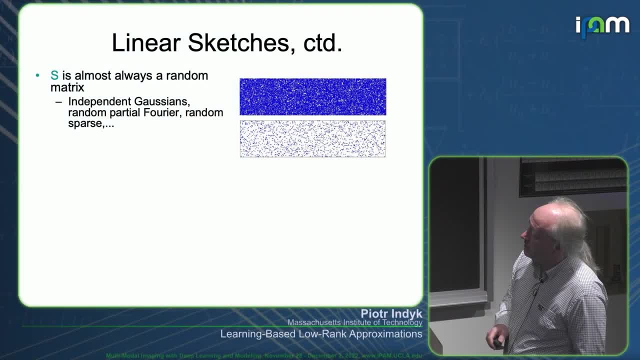 choice of the distributions from which you select those matrices matter. however, in you know all of these applications I mentioned, those matrices are almost always random, And there are reasons for it, right, random matrices are super useful For one, you can easily store them. you can multiply your data by them, right, so they? 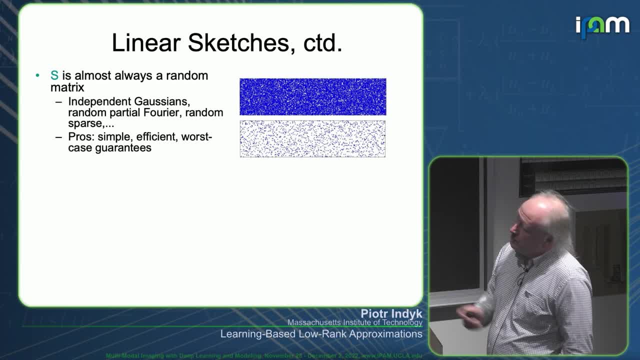 are very efficient And, equally importantly, you have well-scaled guarantees, right, so you know that if you hit your data with a random matrix- right, you have theorems that tell you how much information you lose. okay, So you know that you are not doing something you know at home. 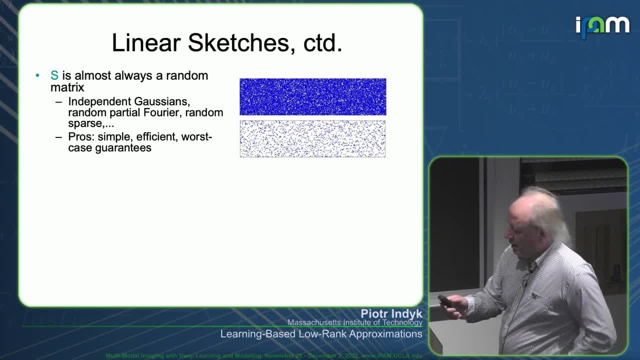 Right. So in a log right you actually have a tail bounce on the, on the probability of error. So these are the good news and this is the reason why they have been so popular. But there are also cons, right, and the main con is that a random matrix, by definition. 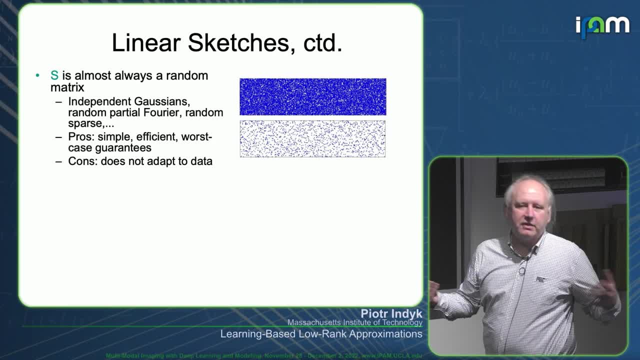 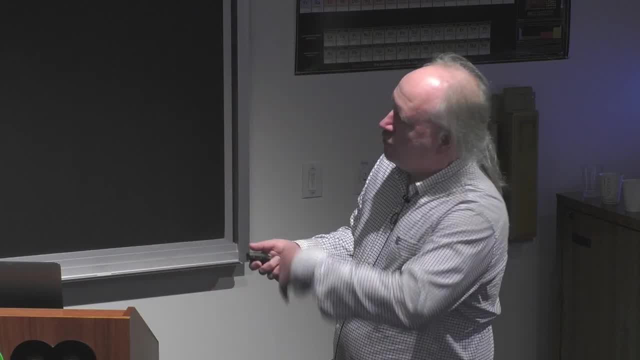 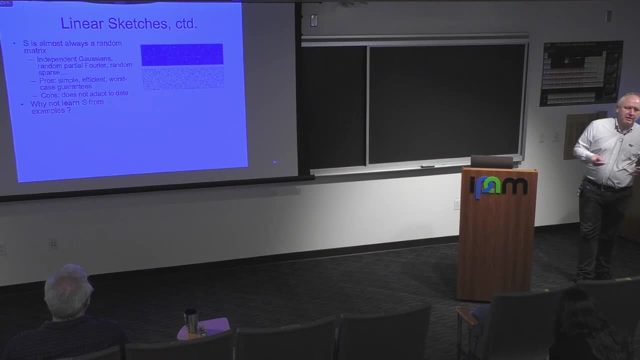 doesn't adapt to data, right, because you know it just doesn't look at the data at all. right, you just generate your Gaussian and without paying attention to what you applied this Gaussian matrix to. So natural question It's: you know, in the applications that I mentioned, you know, can't we just use this? 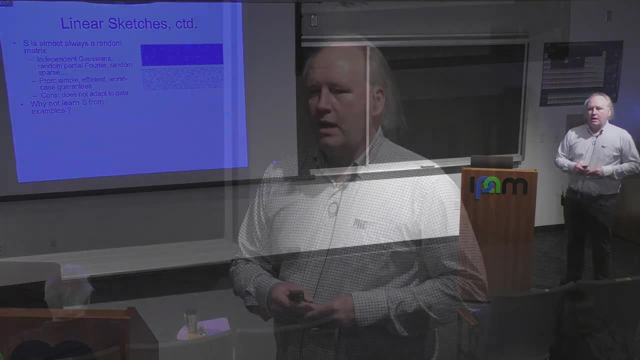 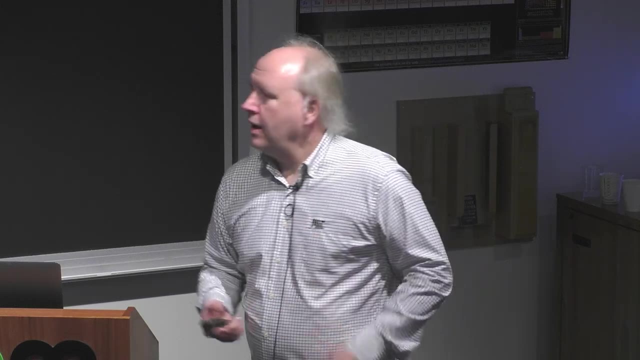 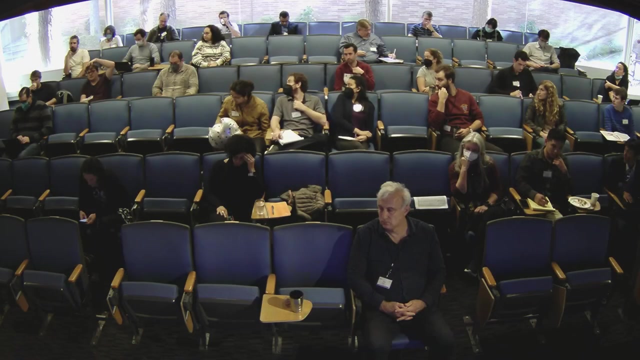 sketch or projection matrix from the data? okay, with the idea that in that case we can actually tailor that matrix to the data distribution right and hopefully improve the reduce the error. And of course- oh yes, Just to clarify- are you talking about like looking at a broad dataset and creating one? 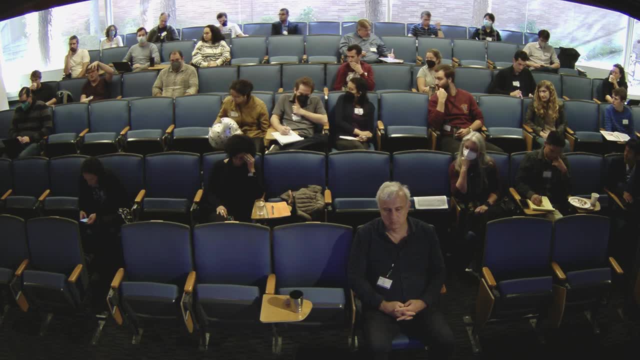 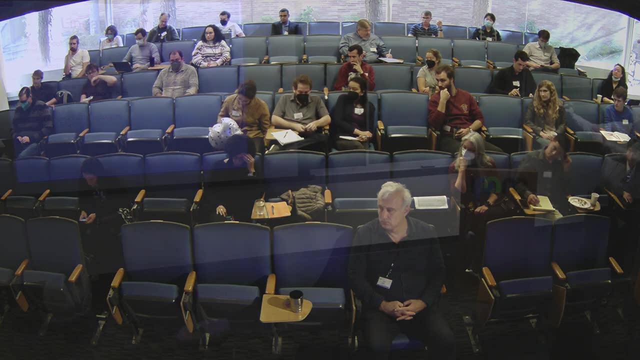 S from that broad dataset, Right? Or are you talking about calculating S on the fly as you gather information about the data you're observing? I see, So I will define the full model in the next slide, but in short, the answer is the first. 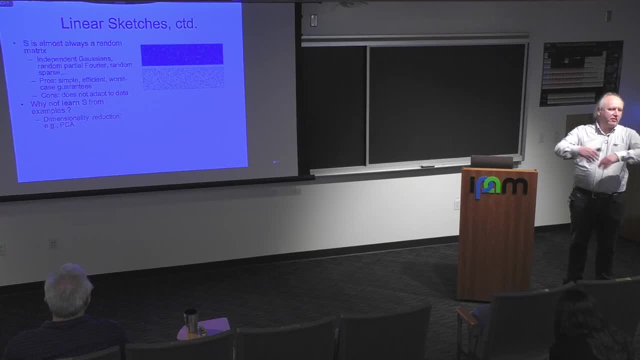 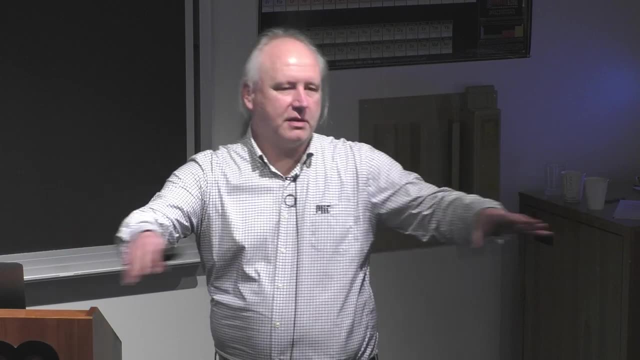 one, right? Yeah, So we'll, you know, we can think that there are lots of many instances and I will look at all of them. come up with some matrix S which is good for those instances, right, and then use this S, you know, from now on, 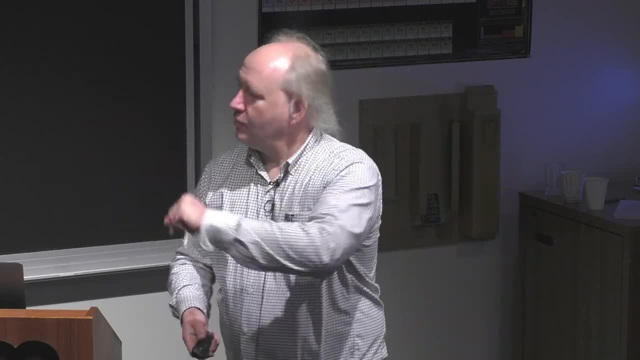 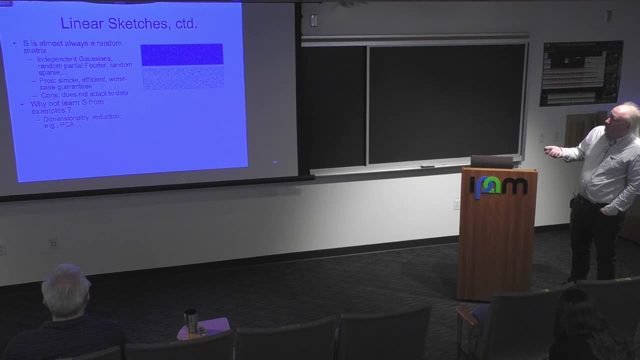 Yeah, And it's a very good question. I will make it more clear in the next slide. Yeah, All right. So you know, of course, this idea is not new, right? In fact, one of the earliest techniques for dimension reduction, PCA. that's exactly what. 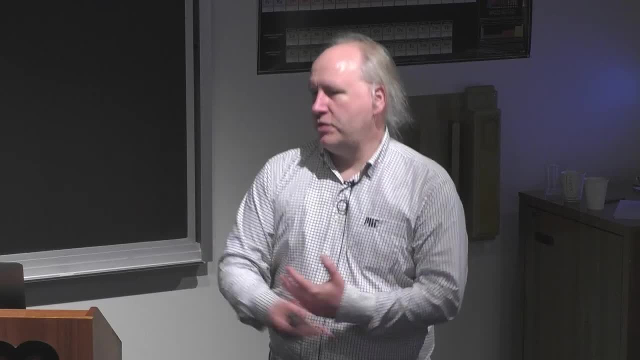 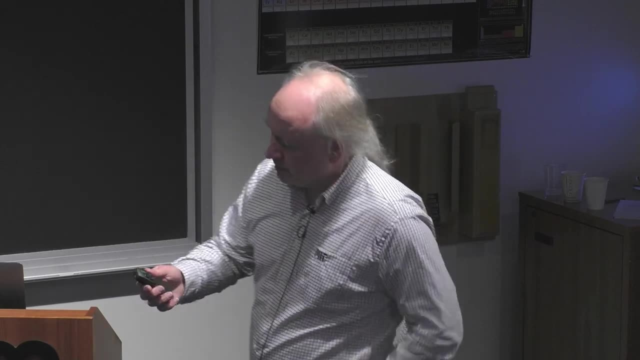 it does right. You know you have a bunch of points and you, based on those points, you try to find the projection right which is, you know, maximally adapted to those points. So the idea is not new. 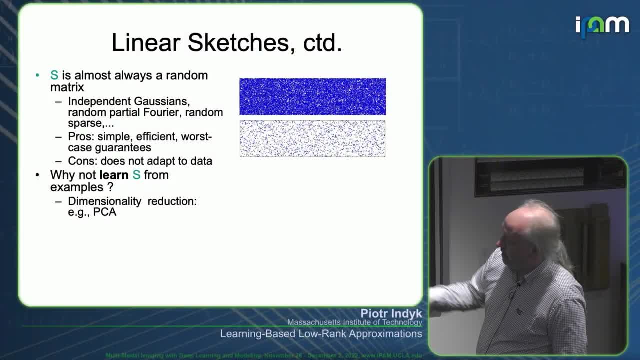 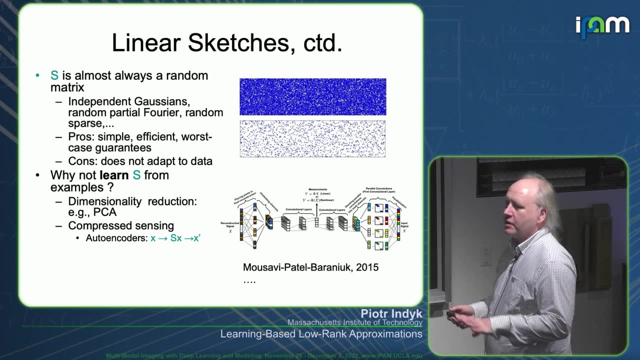 However, in many of the applications I mentioned earlier, this idea of learning or training, the projection matrix, to the best of my knowledge, has been introduced relatively recently. okay, So in particular, to the best of my knowledge, and please correct me if I'm wrong- right. 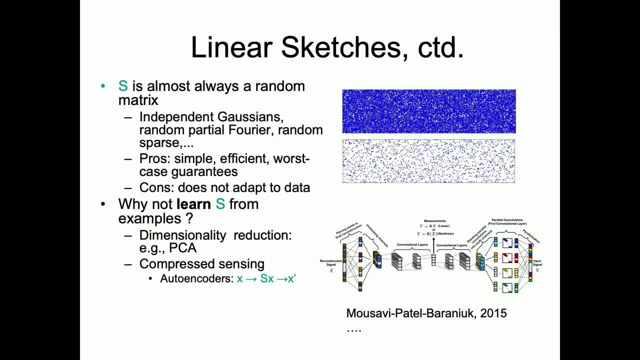 But, to the best of my knowledge, in the area of compressed sensing, this idea first appeared in a very elegant paper by Ali Moussa Patel and Rich Baraniuk from 2015.. And the essence of their paper is a very nice, I would say, interpretation or implementation. 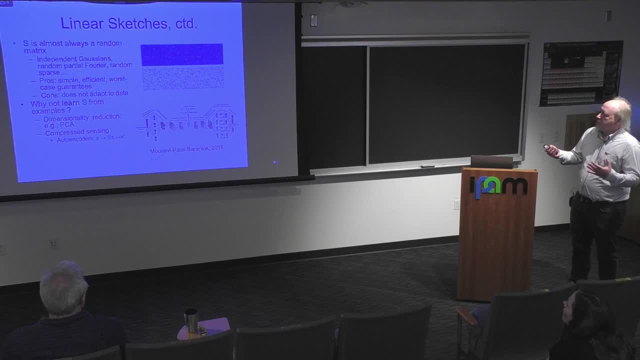 of compressed sensing in the language of a so-called autoencoders. How many people are familiar with autoencoders? Okay, So maybe half right, So the details don't matter. In particular, this picture has a. There are way too many details. 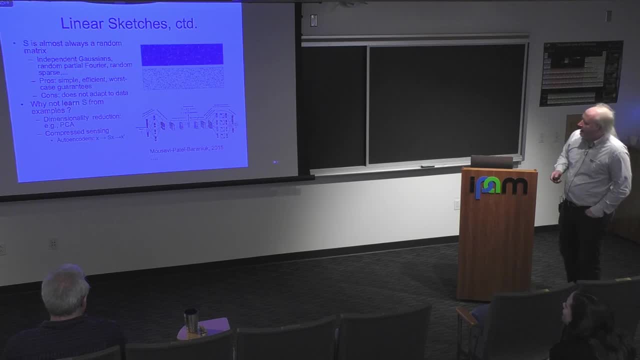 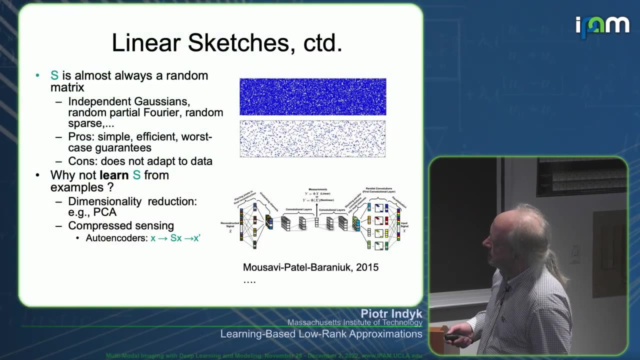 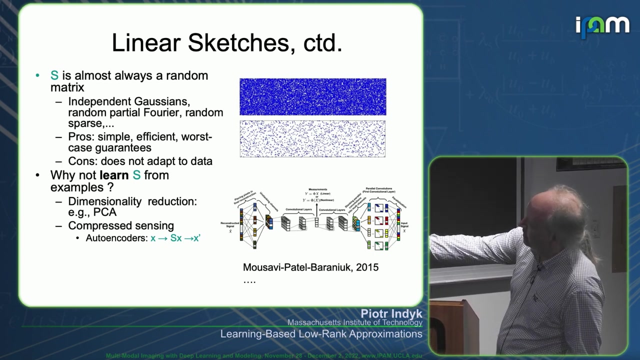 And you probably cannot see them anyway because the font is small. The basic idea of the autoencoder it is, you know, let's say, a neural network which is given an input, some vector x right on the right side. 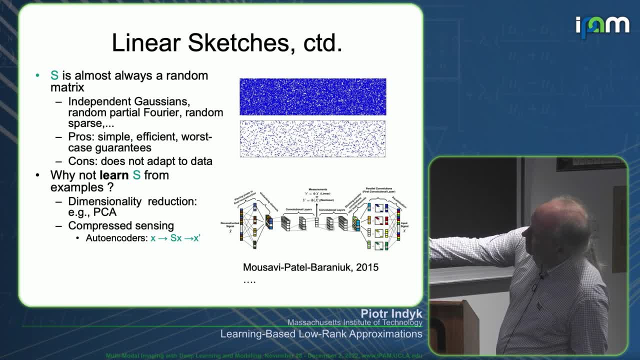 And then this information flows through a bottleneck, like a low-dimensional bottleneck, And at the end this network is supposed to reconstruct this input. And on the left side, okay. And so you train this neural network by presenting it with many inputs and trying to tune the. 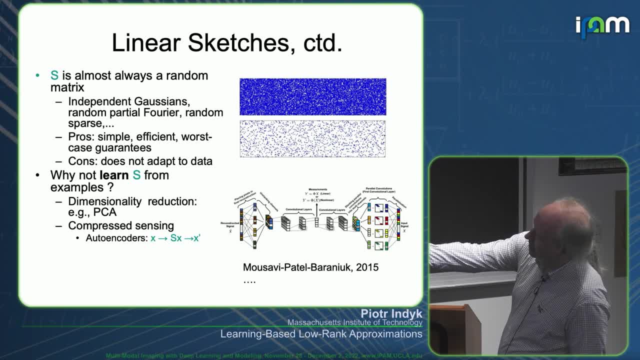 weights so that the error between the input and output is minimized. right, And after you train those weights, you know you can view it as some form of a compression. right, Because you know if you feed it with the input right, then this bottleneck, the information. 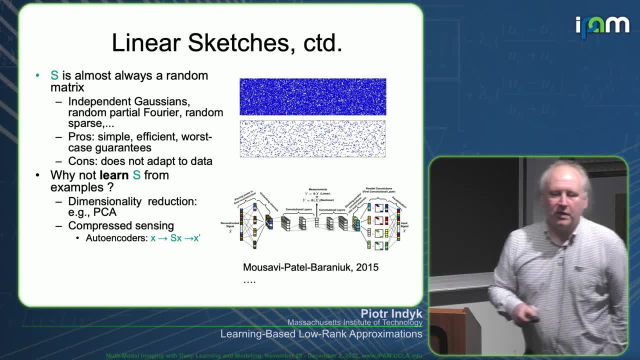 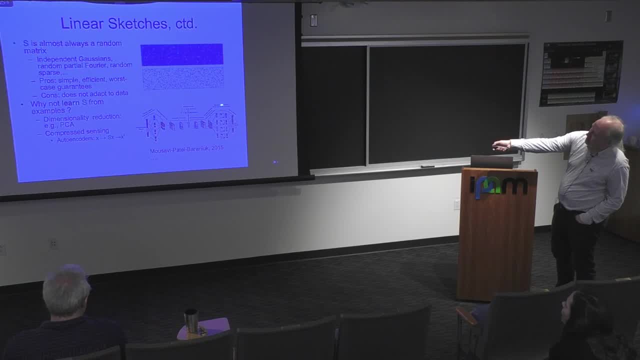 in this bottleneck is the only thing you need to recover output. Okay. So, in particular, if this network on the right-hand side- okay- is just a single layer which only performs a matrix vector product, right then this is essentially a matrix S. 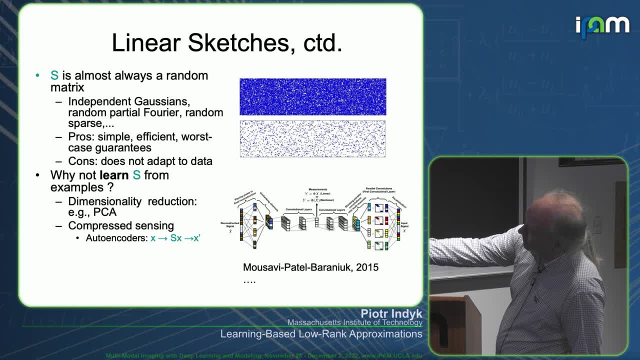 right And you can train the entries. you know the entries of that matrix become weights of this neural network on the side And then you can join them. So you know you can currently train the encoding, the matrix S, as well as the decoder. 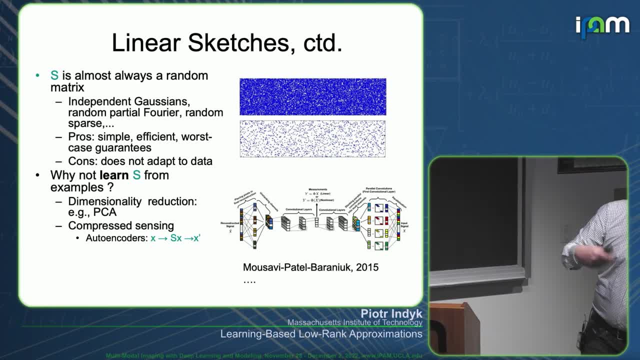 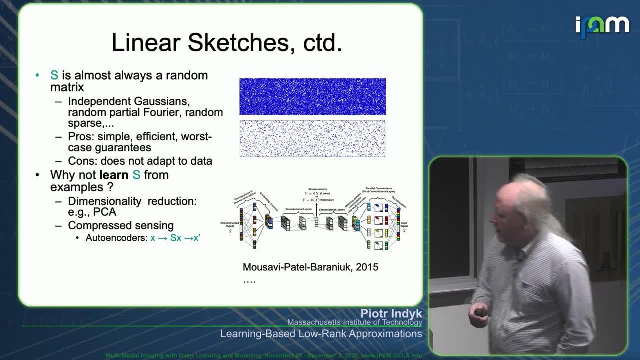 on the left-hand side so that you perform reconstruction from linear projections. Okay, So, this was a very insightful and influential paper And it made several people, including myself, think about you know, like whether one can apply a similar way of thinking to other problems that I use. 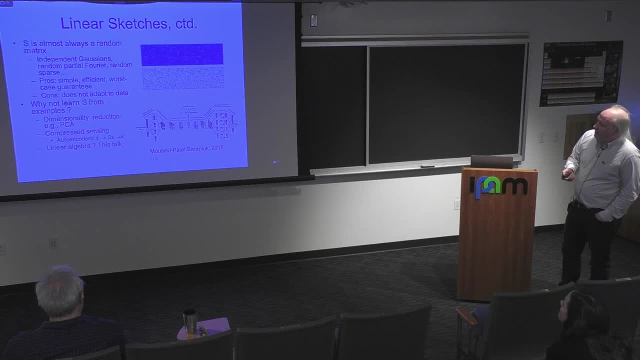 And you know, in this talk I will focus on application of this, you know, approach right of learning matrices from examples to problems in linear algebra. All right, Now linear algebra. you know, of course, it's a huge field. 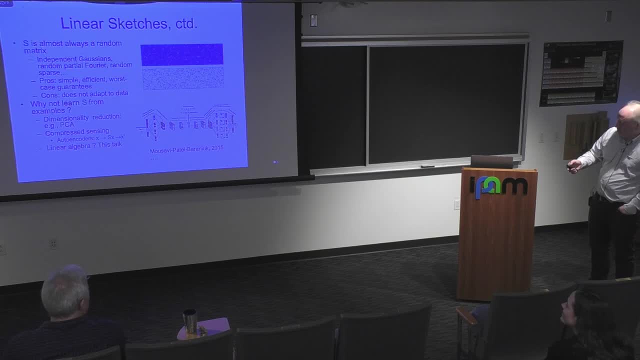 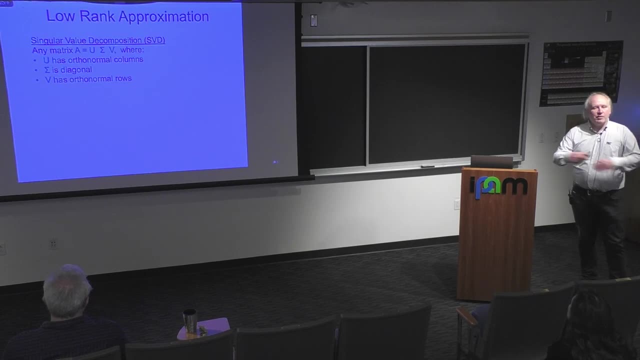 Okay So in this talk I will just focus on one particular problem, which is the problem of the linear algebra. Okay So, linear algebra is a particular problem, which is a low-rank approximation. I'm sure that everybody here knows what a low approximation is and why it is useful. 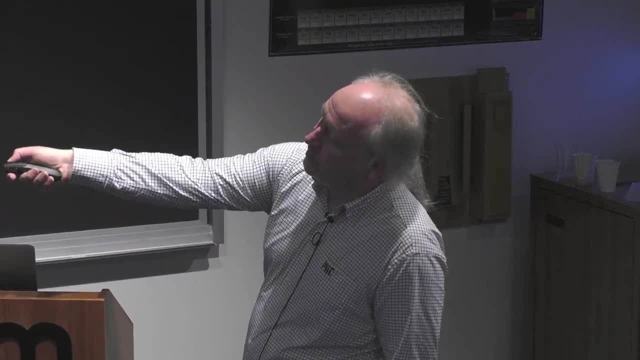 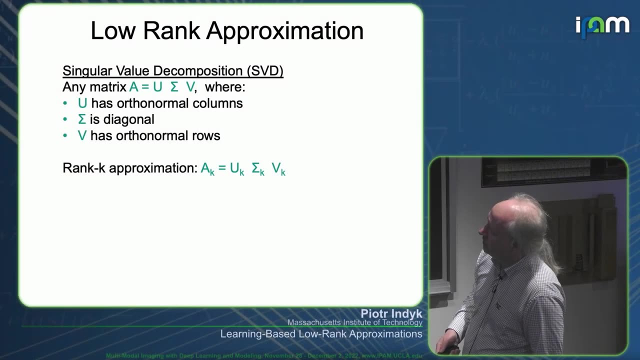 So here- this is just to set up notation Right- We use A to denote the matrix And you know SVD decomposes it. you know into. you know this type of representation In many applications. you know people truncate these applications only to the top set of. 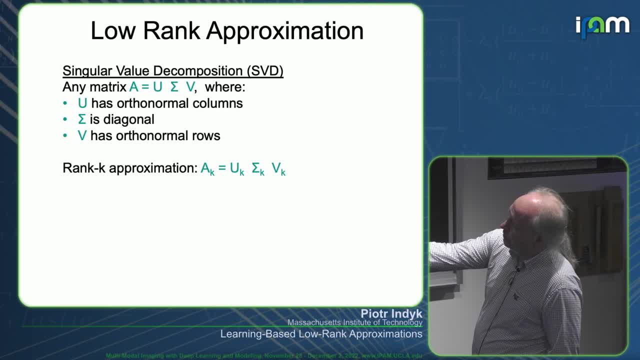 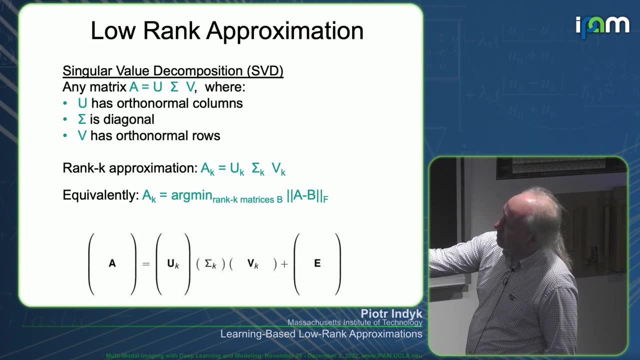 singular values. You know. so here, top, you know, you know, K denotes the number of singular values that we want to approximate this matrix with, And one interpretation of this matrix here is that it minimizes over all rank B rank. 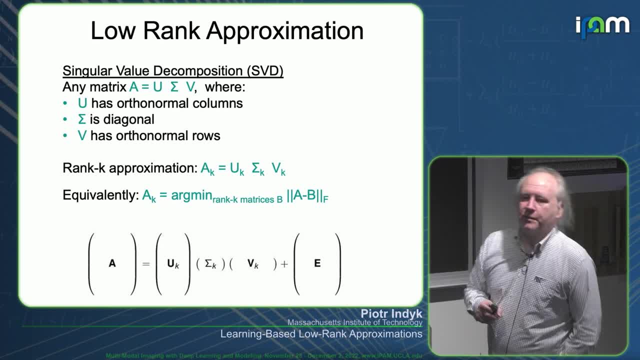 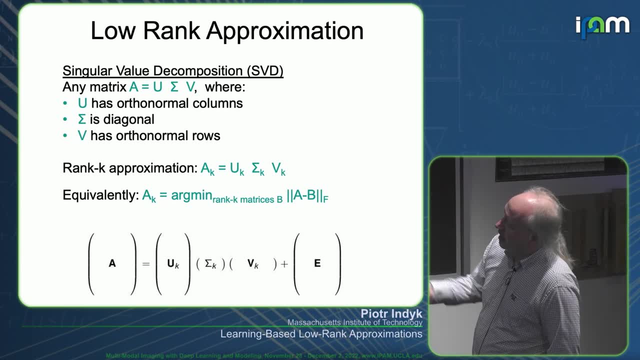 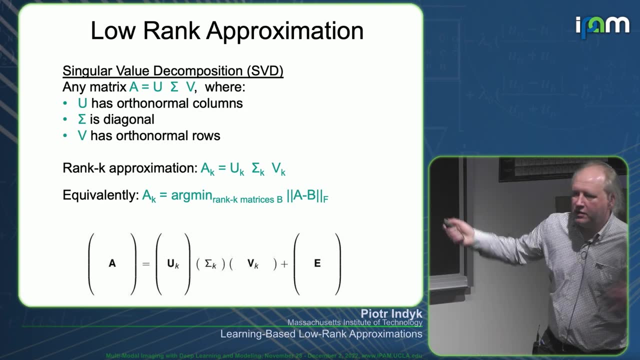 K matrices: the Frobenius distance to the original matrix. Okay, So this is the error- approximation error- that we don't care. Okay, So if we truncate this representation, if we restrict this to only top K singular values, Okay, 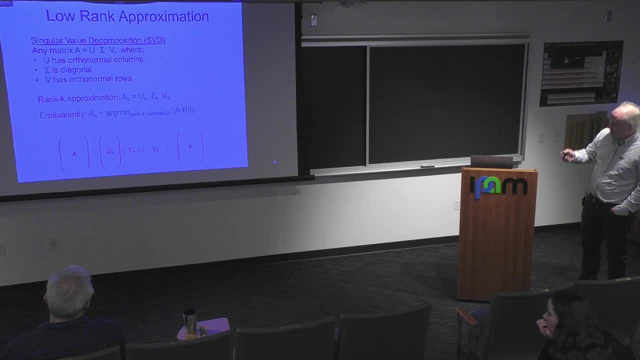 So nothing new here. This is just the definition, All right. So of course this is. you know it's hard to you know overstate how important this problem is, And lots of very efficient algorithms, libraries, implementation have been done. 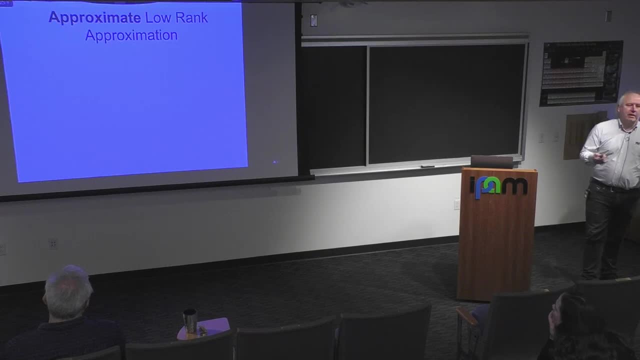 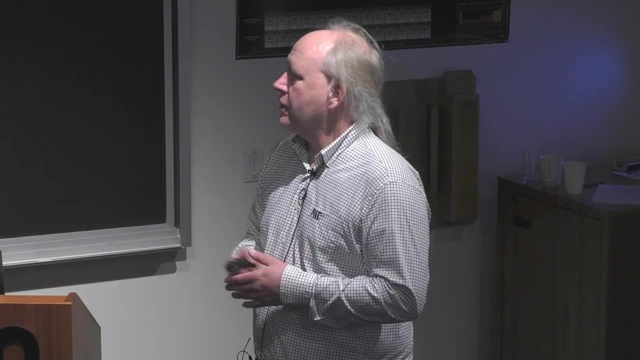 Still, you know this problem does not have a linear time solution, Right, And you know typically, to the best of my knowledge, the algorithms used, you know, let's say for matrices N by N, running time and cube. 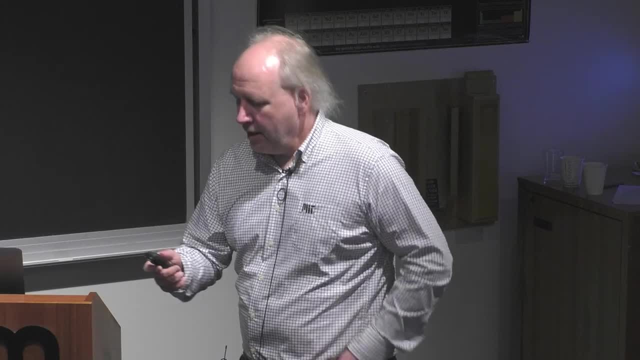 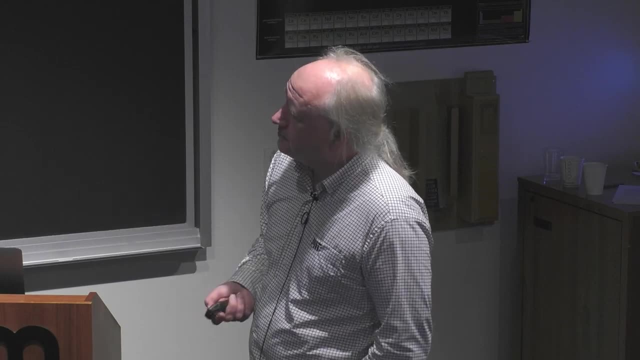 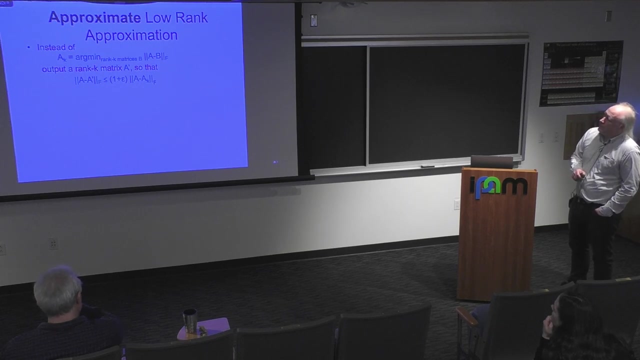 Right, You can get it a little bit faster using the Strassen method, Right, But this is often too large in many applications, especially when the matrices are sparse, Right. So because of that, especially over the last 15 years or so, people developed lots of approximate. 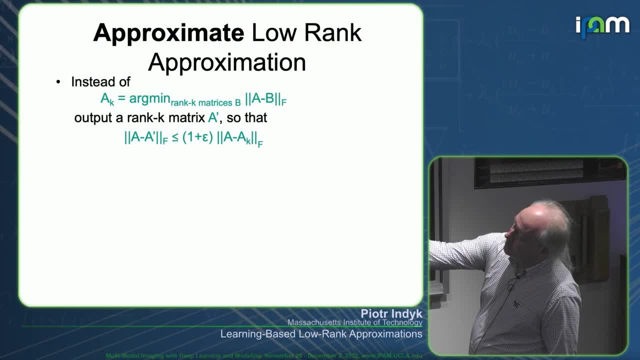 algorithms for this problem. And here the approximation is a respect to the Frobenius error, Right? So instead of getting the optimal matrix, you know, the algorithm that people developed, you know, give you error which is 1 plus epsilon times the optimal error. 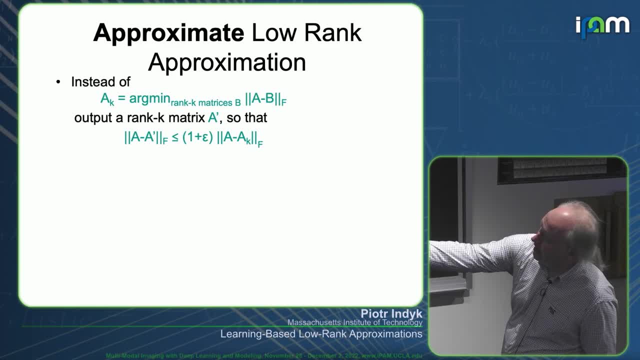 Right, So this epsilon times this tail is the cost of using those faster algorithms, Right, And there is of course a trade-off between the approximation and the running time And of course there is a particular problem. Okay. 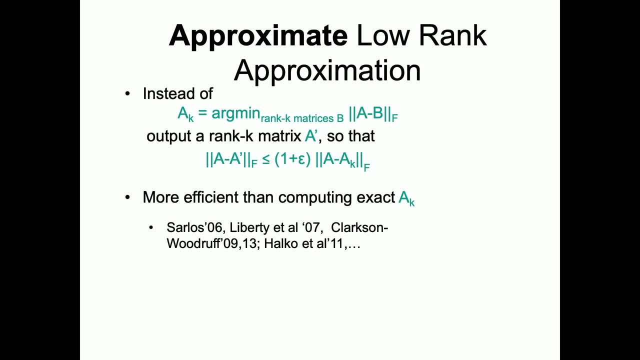 So the reason people are doing it is because you can solve this problem for a reasonable value of epsilon more efficiently than computing the exact decomposition And, starting from the work of Sarlosz Liberty in the mid odds, lots of such algorithms have been developed. 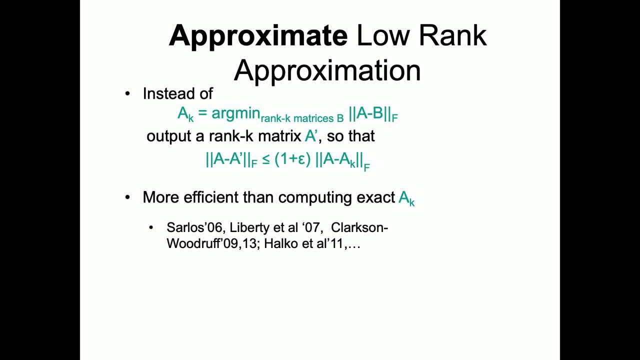 I'm not going to, you know like state the results, because that's actually a big field right now, Right, But you know there is a survey by David Woodruff which you know gives a very nice overview of the state of the art in this area. 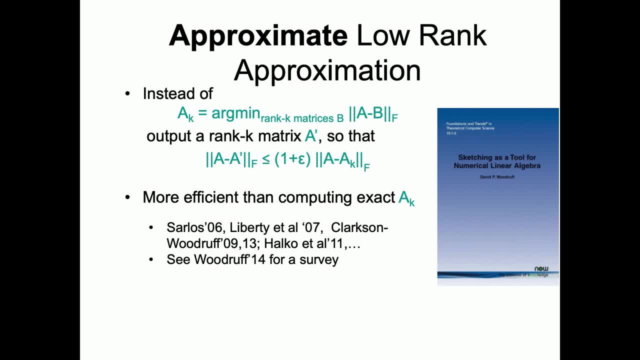 But just to give an example, you know, for natural values of, let's say, parameter k, you can compute such an approximation in time, which is a linear number of no zeros of the matrix Right, Which is particularly good if your matrix is relatively sparse. 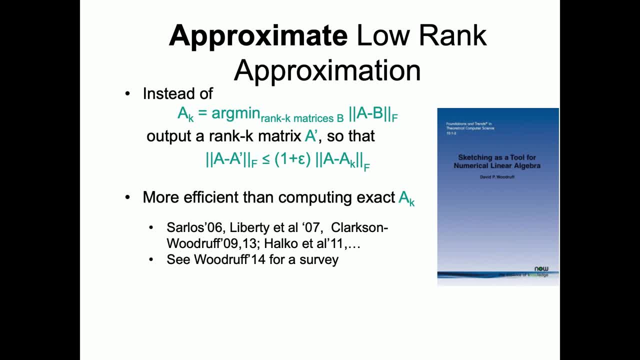 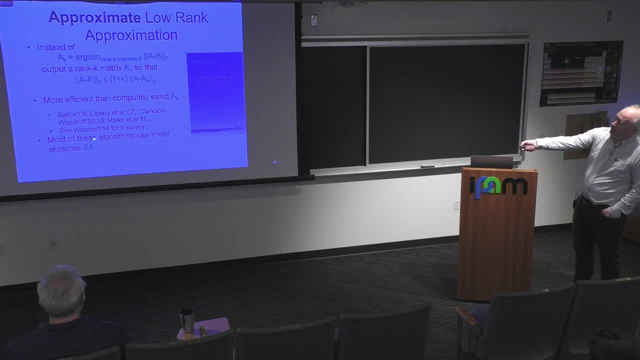 Right, And if you want to learn more about it, you know this is a very good introduction. All right, And you know, perhaps not surprisingly, most of these algorithms are using the sketching approach. You know the first thing they do, and sometimes the second and the third is, you know, to. 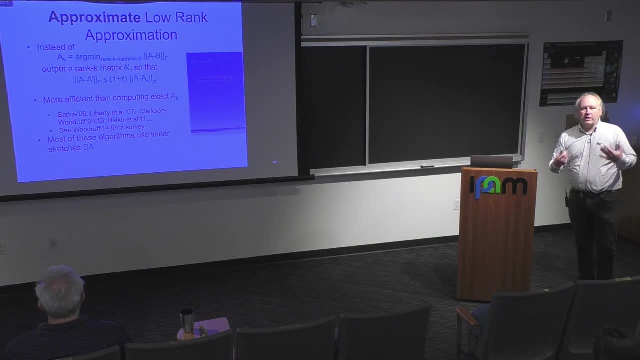 hit the input matrix with the sketching matrix Right And then perform the computation over the sketch Right. So this is one of the sources for their efficiency And for efficiency reasons, these matrices are typically either partial, Fourier Right, So we can compute this projection using FFT, or, you know, they are sparse. 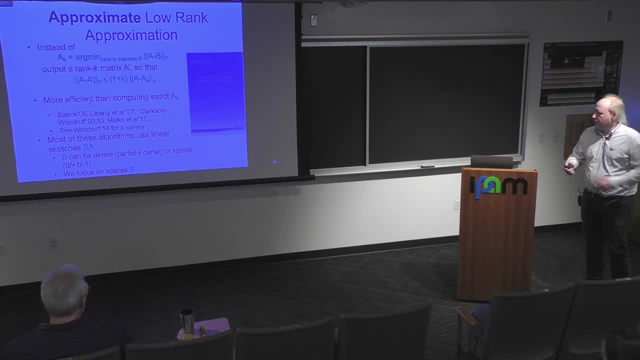 In this talk I'll focus on sparse matrices, Right? So you know very sparse matrices, you know, which still preserve the important information about the matrix after the projection. All right, So? So this is the type of algorithms that will try to merge or refine using machine learning. 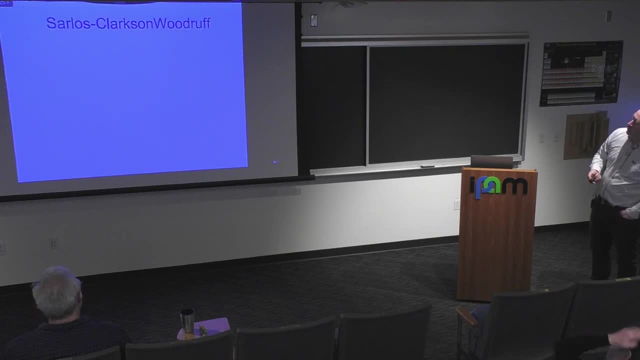 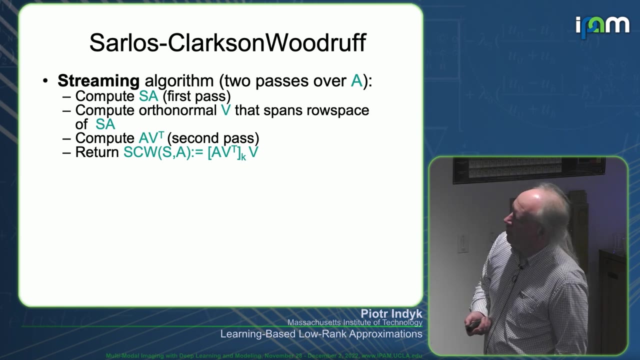 methods. Okay, And before I get to how to do it, let me just give an example of an algorithm. So this is the algorithm that we'll focus on in this talk. The details of the algorithm are not necessarily that important, Right? 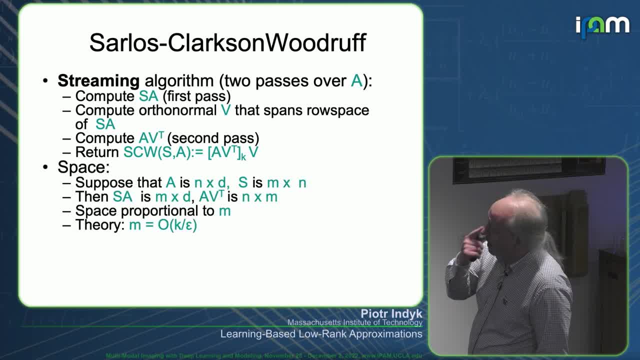 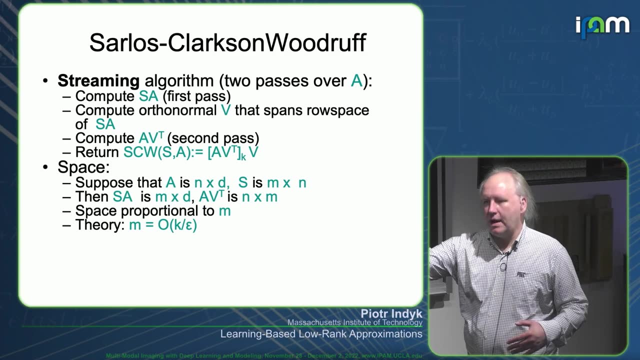 I'm just putting here for completeness What. Okay, So what matters is that this is one of those algorithms that use very little space. Okay, So this algorithm is called a streaming algorithm, Right? Which means that it operates by performing two passes, in this particular case, over your. 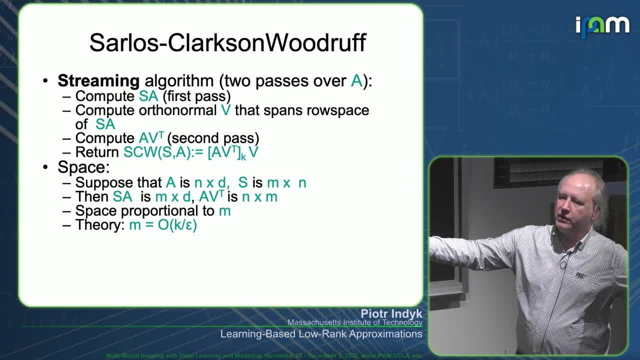 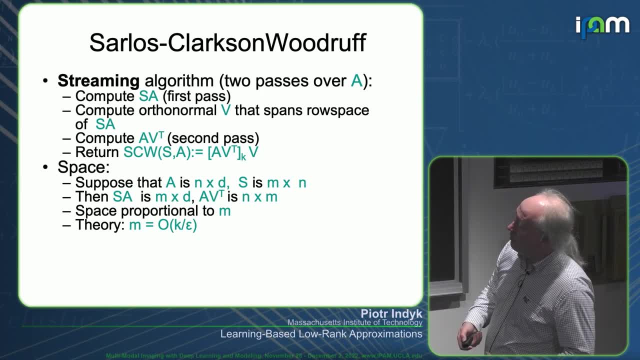 input matrix, Right, Which this matrix can be stored somewhere on disk. Okay, And you know, instead of storing this matrix in your main memory, Right, It passes over this matrix stored over the disk, And what you stored in your memory is only the sketched version. 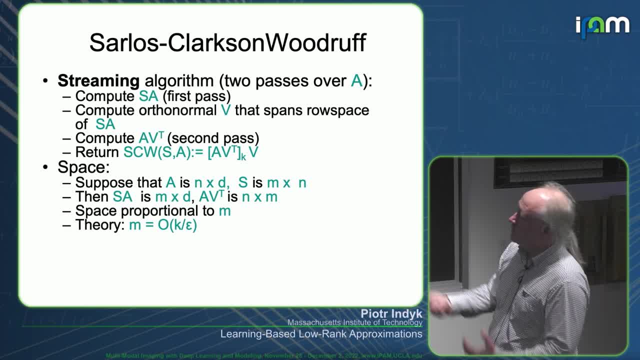 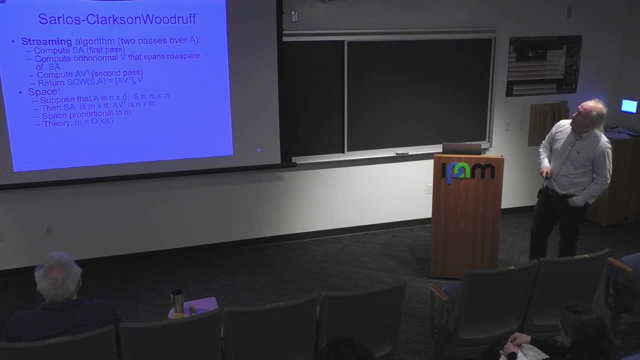 Right, So it requires. the benefit of this algorithm is that it uses much less space than an algorithm which would store the whole matrix in the main memory. Okay, And basically, the efficiency of this algorithm is strongly related to the number of rows of this sketch matrix. S Right, 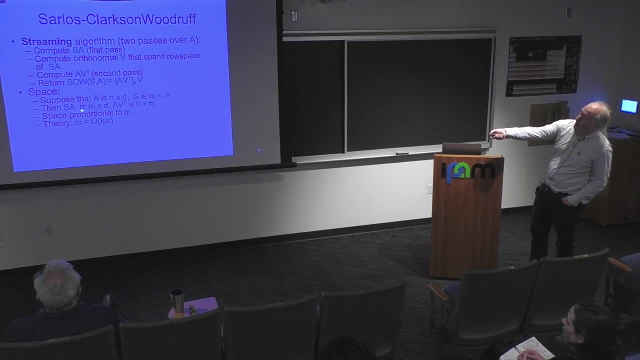 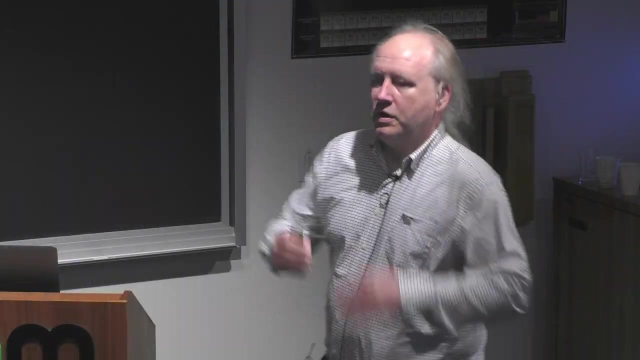 Because essentially the space it is using is M times D plus N. D and N are the dimensions of the original matrix Right. So in other words, the space used by this algorithm is proportional to M, Right, The number of rows in the sketch matrix. 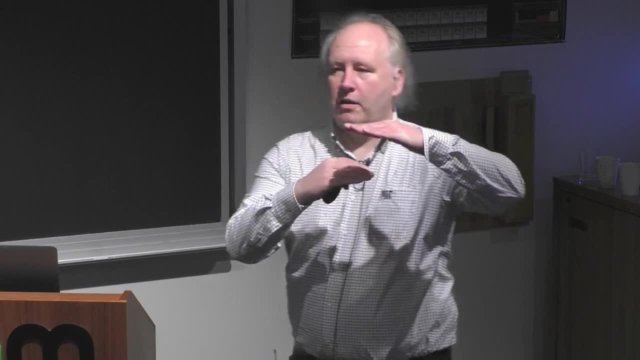 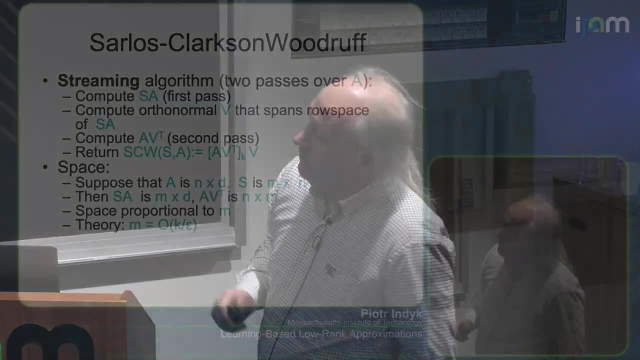 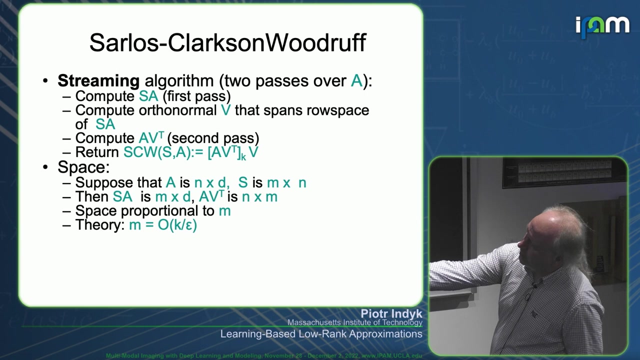 So the shorter we can get this matrix to be, the more space efficient. the algorithm is Okay And the theoretical result shows that If you want to get K rank, K approximation with an error epsilon, you can set M to be this much. 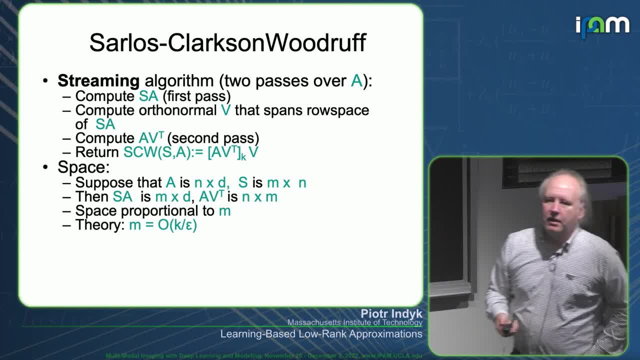 And the algorithm is guaranteed to give you, you know, epsilon error with some decent probability. Okay, So this is the theoretical guarantee for this algorithm if the matrix A is not chosen to be random Right And if the random matrix does the job here. 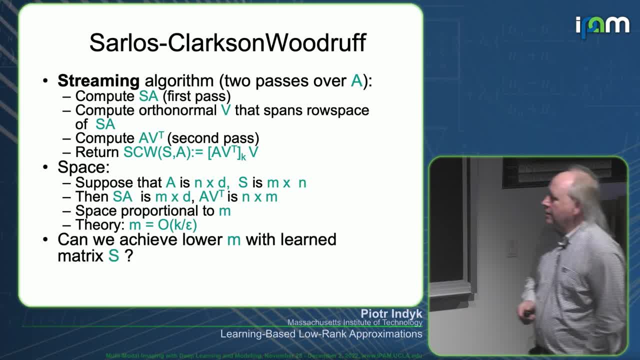 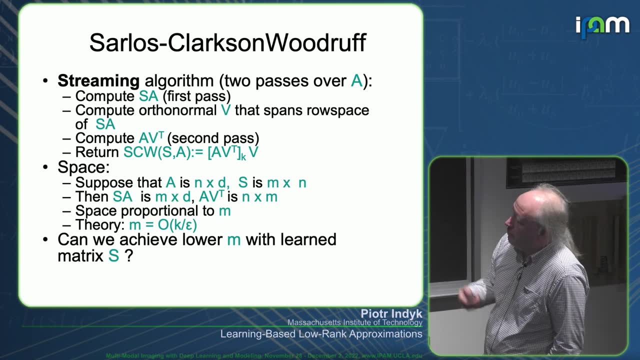 All right. so the main question in this talk is: can we improve over this Right? So this is a theoretical bound. You know, can we. but even in practice, you know, can we achieve a better performance? meaning, can we live with smaller M if, instead of using a random matrix S, you know we somehow. 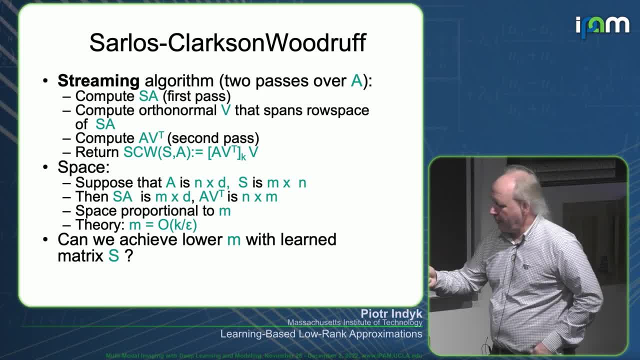 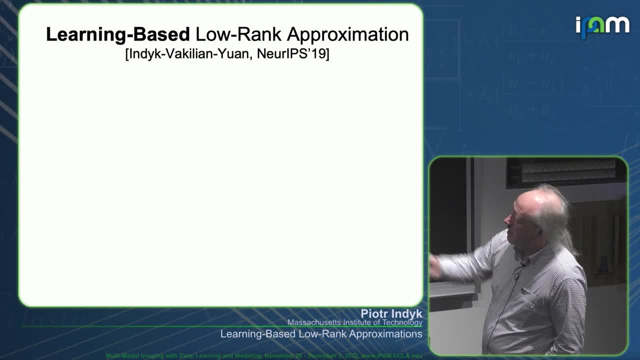 it using the input data? Okay, and so that's exactly the question that we set to answer in our first work on this topic in 2019.. So the framework, and this is like the, the formal framework, right? I guess it was not the next slide, it was. 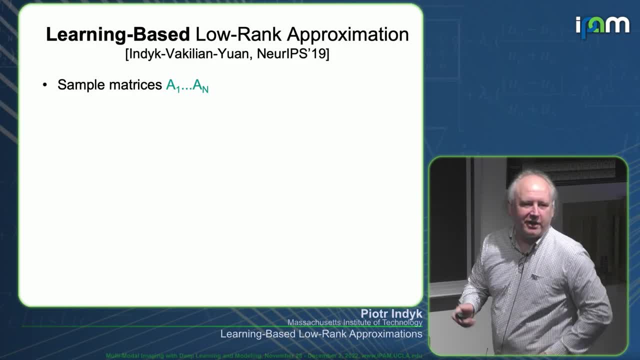 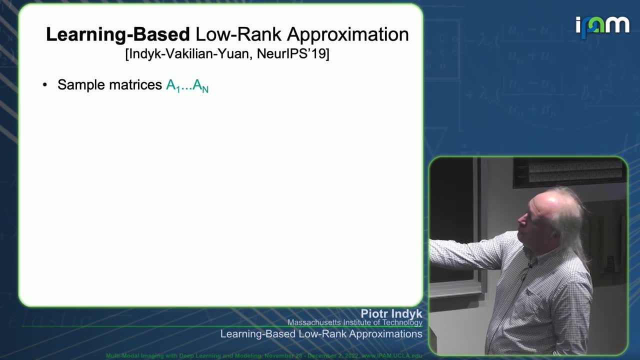 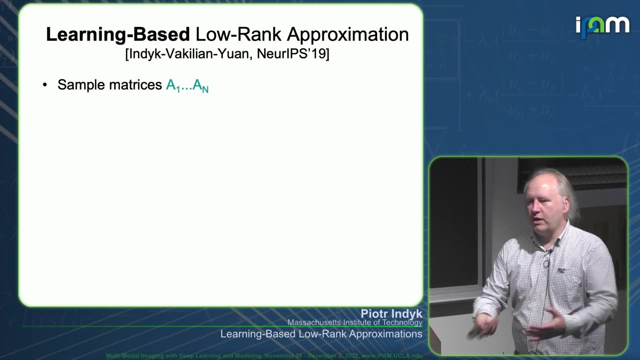 next few slides, right, but you know, hopefully after this slide it will be clear, right? yeah, So the framework is that we sample. we assume that we have an access to a bunch of inputs to this problem, right? so this is not a setting, it's not a one-shot setting. right that you are given a matrix, you compute. 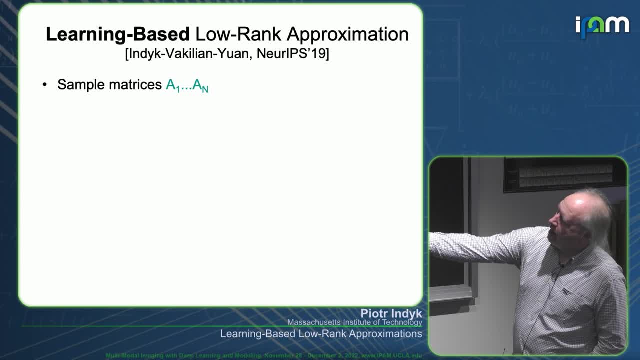 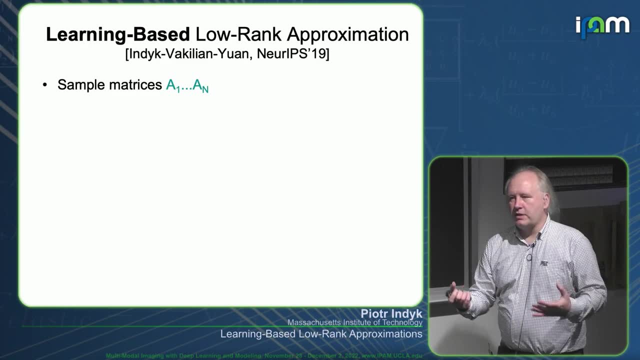 something. it's a setting where you are first given a collection of matrices that come from the same distribution and then you perform some computation, do some pre-processing and you construct a very efficient low-rank approximation algorithm. and then you perform some computation, do some pre-processing and 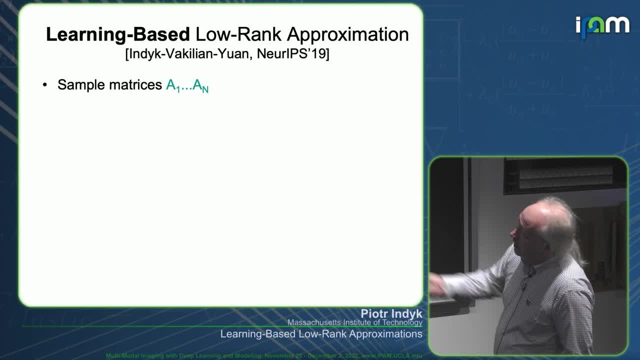 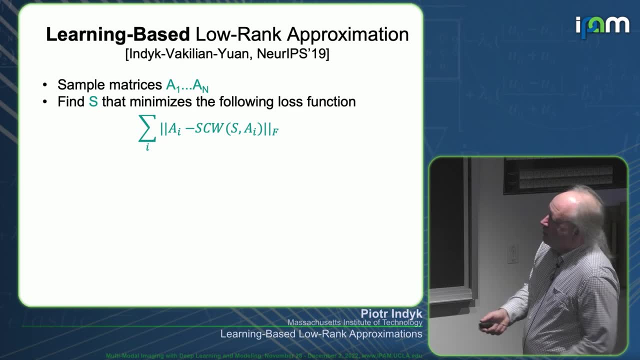 then you perform some computation, do some pre-processing and then you perform some that you can use from that one. Okay, so we take a bunch of sample matrices and that you can use from that one. Okay, so we take a bunch of sample matrices and you know, the only three parameters in those are low-rank sketching based. 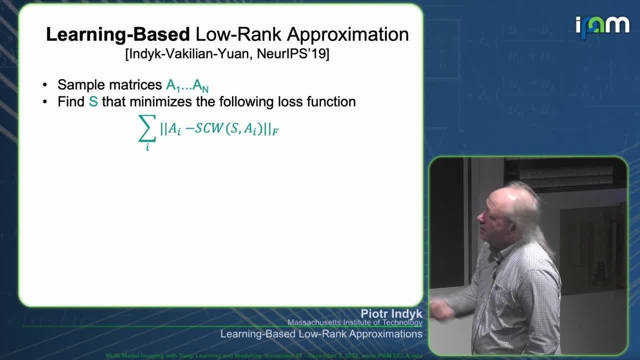 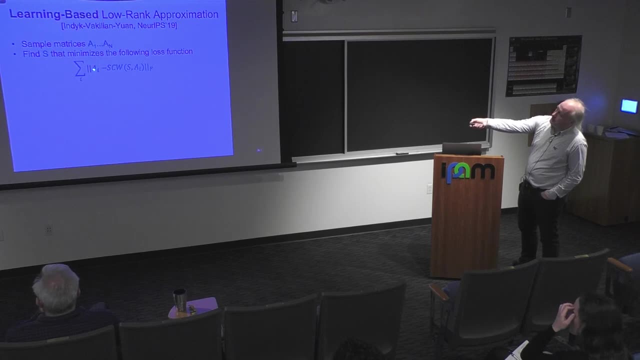 algorithms. is the matrix S right? so we learn the some matrix S by optimizing the empirical error, right? so this is the sum over all the training matrices and of the difference between the actual matrix and whatever the previous low-rank approximation algorithm gives us, given AI as an input. 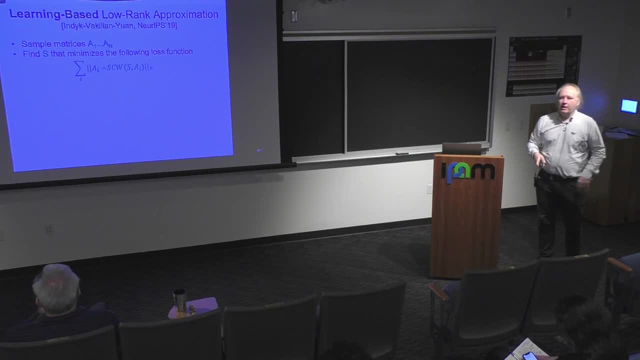 and S as the sketching matrix. So basically we want to take S to minimize this empirical error with respect to the prior sample matrices which we use to train this matrix S And once we train it then we use S in all the future computation. 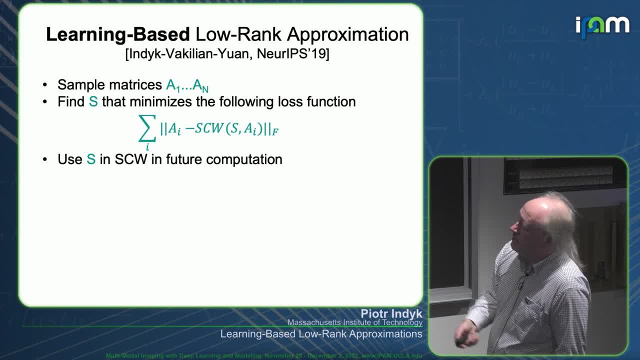 So this is essentially the basic idea behind the approach. Of course, problems like that are always more complicated than this simple statement. There are lots of details. So some of the details, some of the details that we had to overcome in order to make this happen. 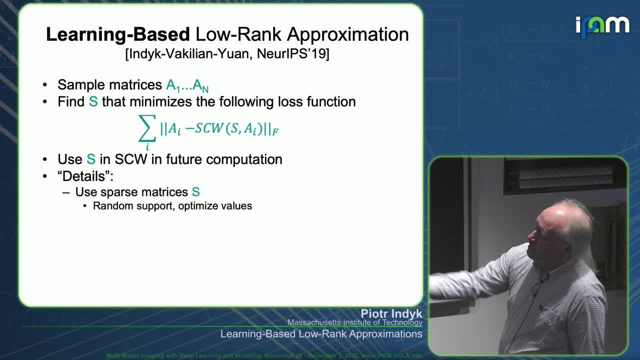 are as follows: right, So for starters, as I mentioned, we use a sparse matrices S which basically look like this: They have only one no-zero per column And it's relatively easy to optimize over the values of those no-zeros. 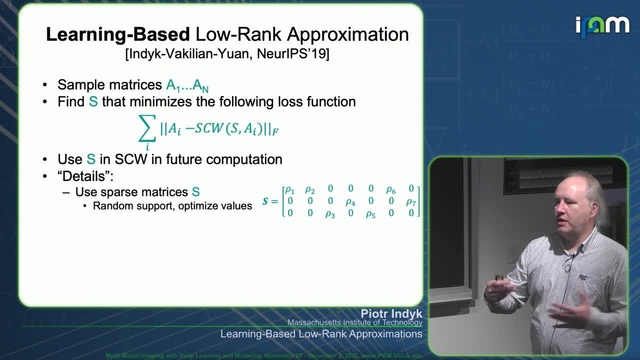 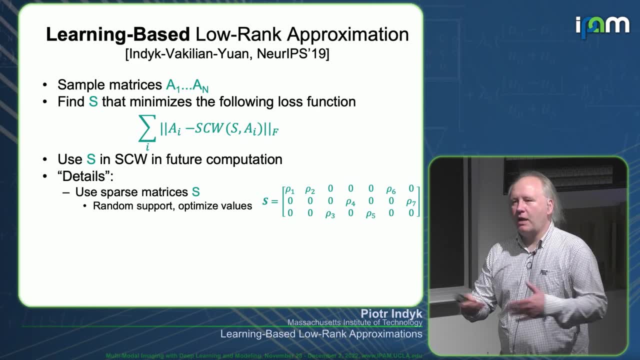 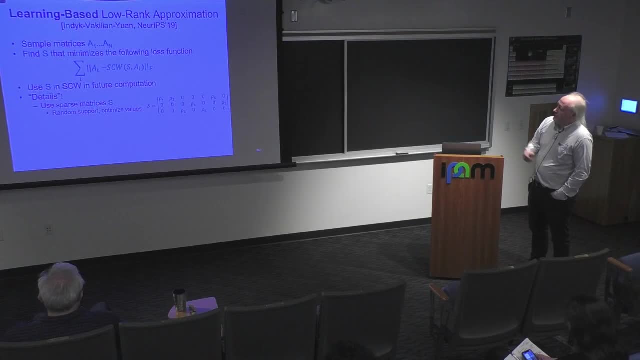 but optimizing over locations it's much more difficult, right? Because you know it becomes a combinatorial optimization problem, right? As opposed to continuous right? So basically, we kind of introduce a hack, meaning that the locations are still random, right? 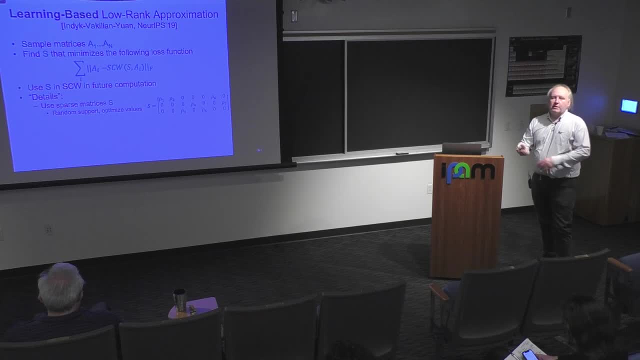 As in the original Sarlow SCW algorithm. but we optimize only the values right, So it's like a partial optimization of this right. We only optimize conditioned on the no-zero entries of S being, you know, being fixed as before. 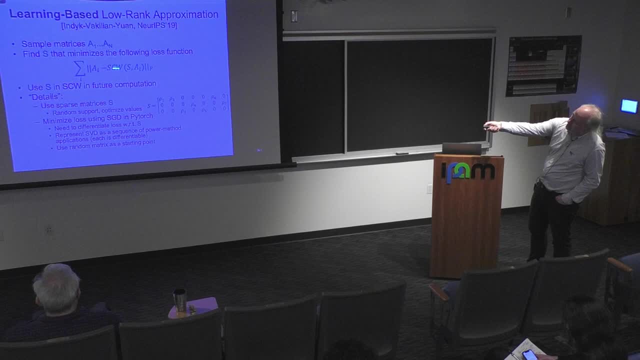 So that's one thing. Now, the other thing is that you know, as you can imagine, you know this is a pretty hard problem to optimize. It's highly non-convex, high-dimensional right, So we are not able to optimize it to, you know exactly. 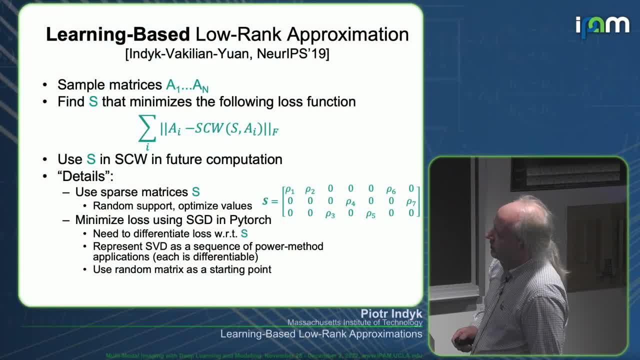 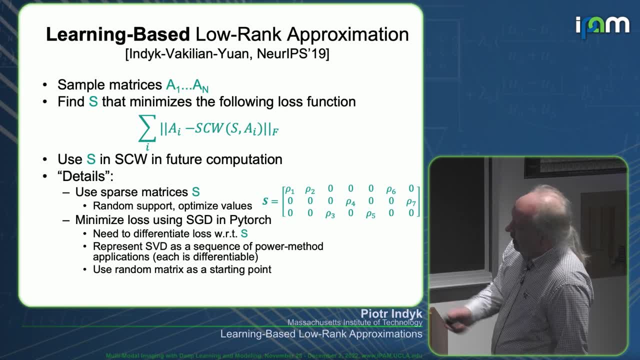 Instead, you know, we do what people do in deep learning literature, right? We just run stochastic gradient, descent, right? So we basically find some local optimum And leave with that. Now, for this to happen, we need to be able to differentiate this loss. 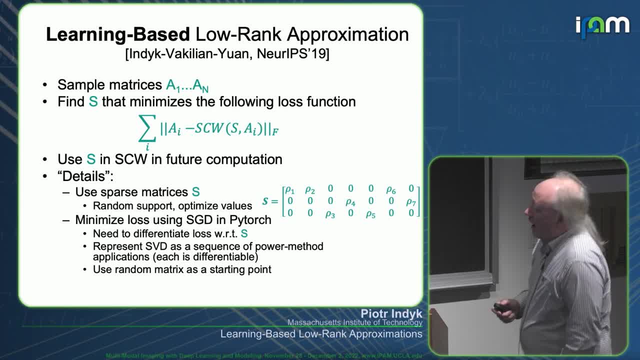 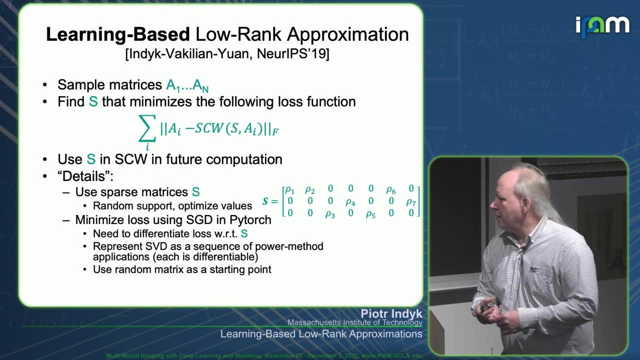 with respect to the matrix S And in our original paper we didn't know how to differentiate SGD in the system. So basically we compile SVD, you know like, as a sequence of basically we implemented SVD as a power method, right. 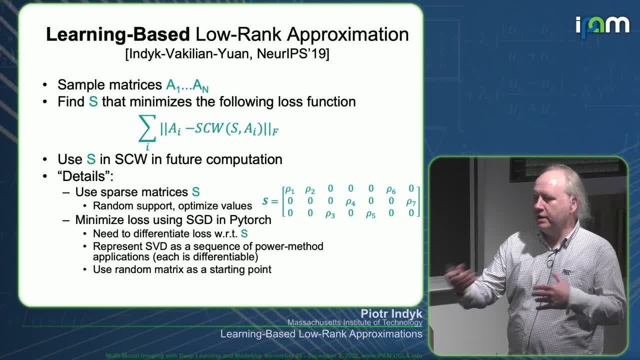 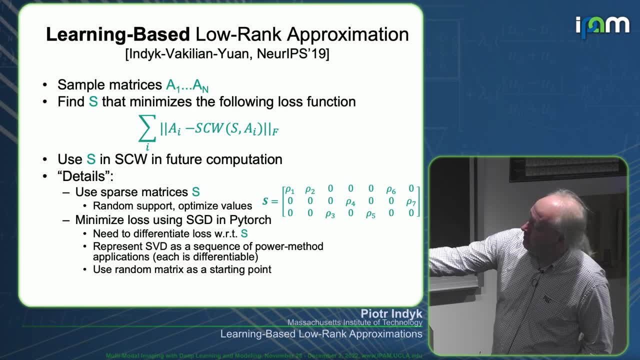 And then we don't have. we don't have to, we only have to differentiate the matrix vector, multiplications, right, Which is already something that the system supports. I believe that now you know SVD, it can be differentiated directly in the system. 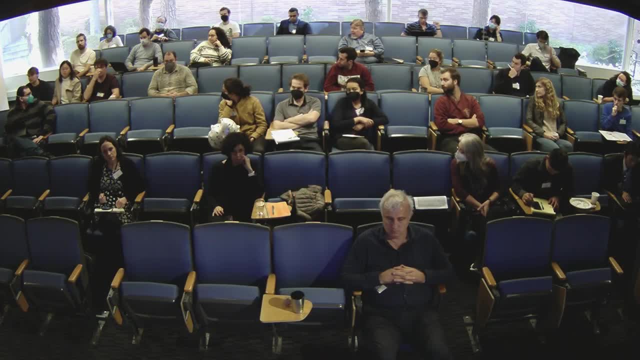 Yes, If I understand correctly, you pick a random support for S and then you optimize for the values. but Yes, There's another strategy where you put, like a sparsity constraint on S in your optimization of the like loss function. 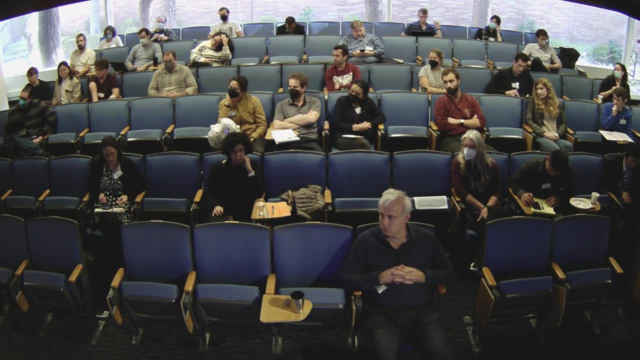 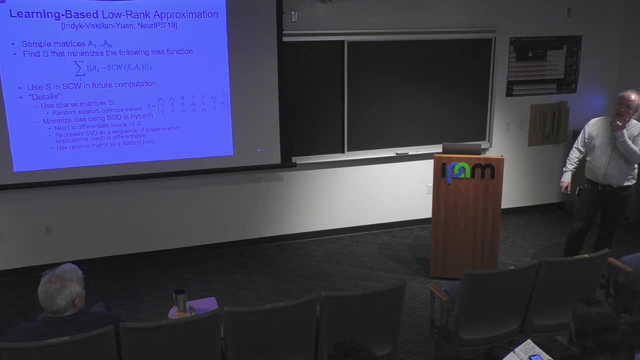 Right. Do you have a reason why you pick one versus the other? Well, we picked this one because it was simpler to start from. There is another follow-up paper that we mentioned earlier that also optimizes over support. It does something different than what you suggested. 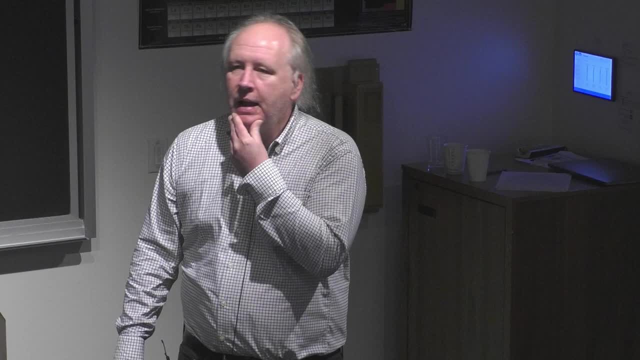 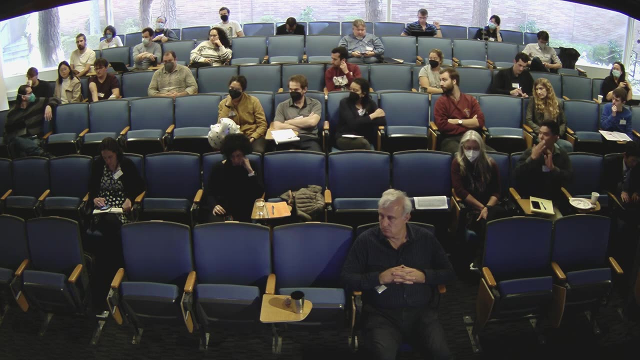 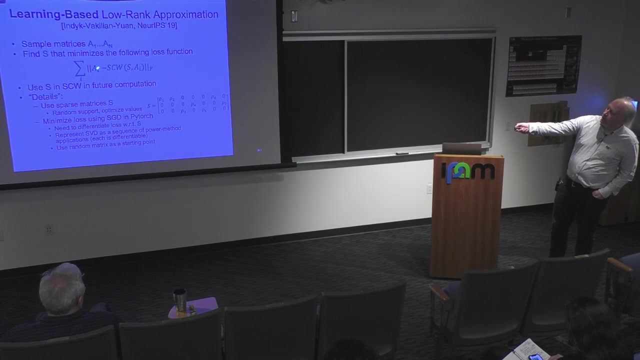 Yeah, I guess the main difficulty- You're saying that picking a random support is not like affecting the ability to like do the computation we want with S Well, so what it means is that we might not be getting S, which is as fixed. 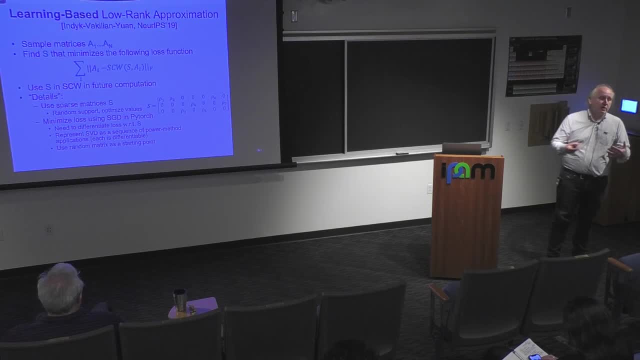 but if it's going to increase his output size, yes, we're going to increase the option value, Which is as good as possible, right? So potentially it could affect things by a lot. We just don't know because we never find found the the optimum right. 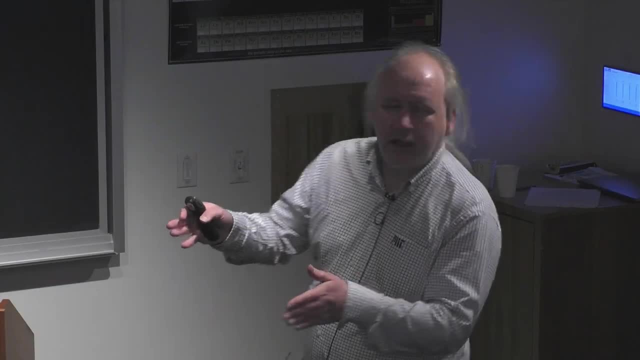 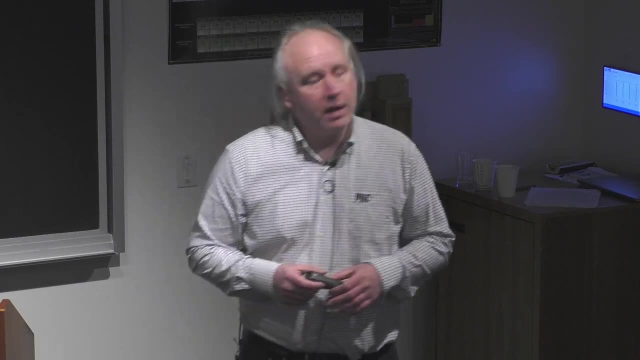 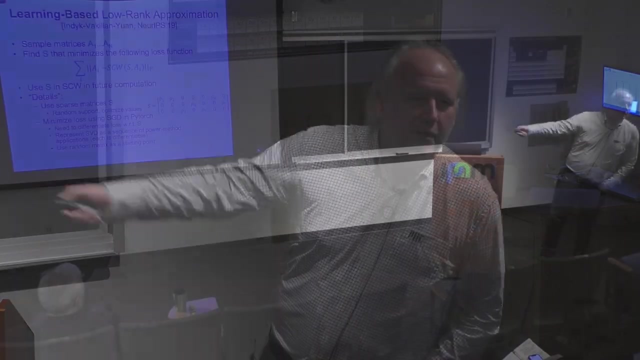 Right, So you are thinking about Putting like a zero constraint or a one constraint? Yeah, so we didn't try it. it's a. it's a. it's a very interesting idea. Yeah, we, it's also a natural idea. I guess we in this paper, We just wanted to start from something, right? 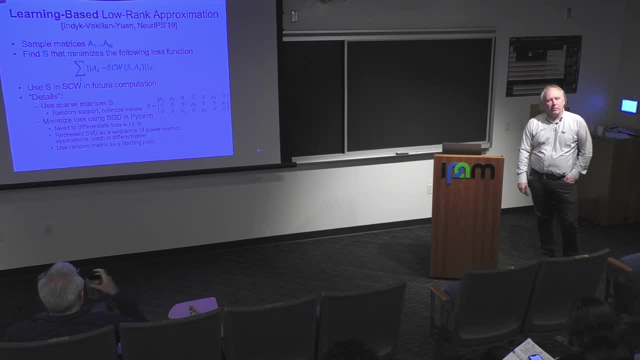 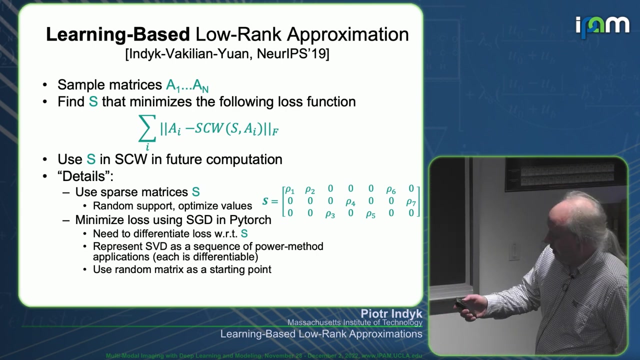 but it's, it's a very, very good point that we could just add a one musician right and- and We know, hope that in this setting it will also reduce the sparsity right. There was a question or all right, All right, so Right, and basically this and this, we are using our graded descent. we have to step from somewhere. 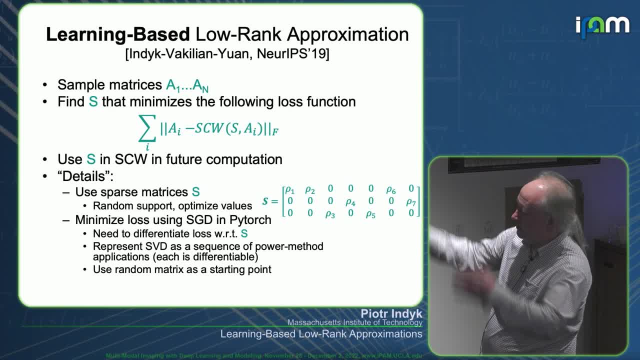 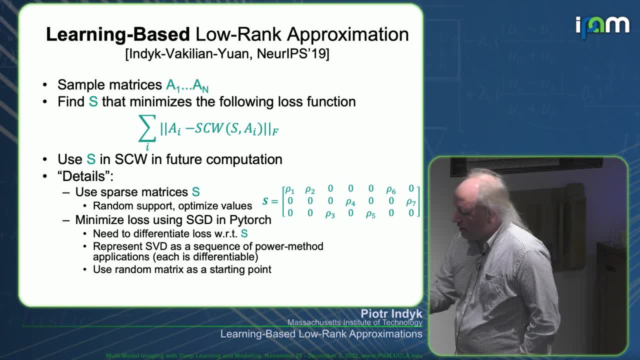 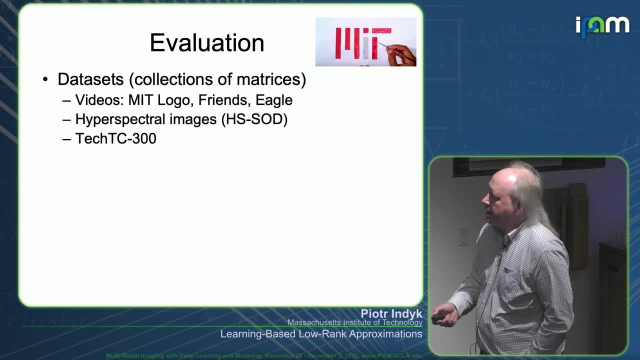 So We just use random matrix as a starting point, right, and just do a graded descent, you know, to minimize this empirical error. So, because the the main question here is empirical, you know, does this work? And to answer this question, you know we have to focus on a particular class of our matrices. 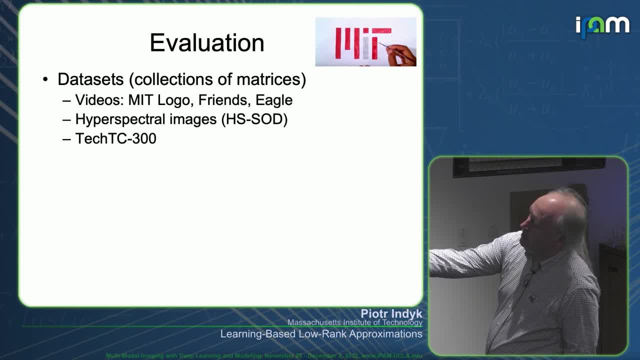 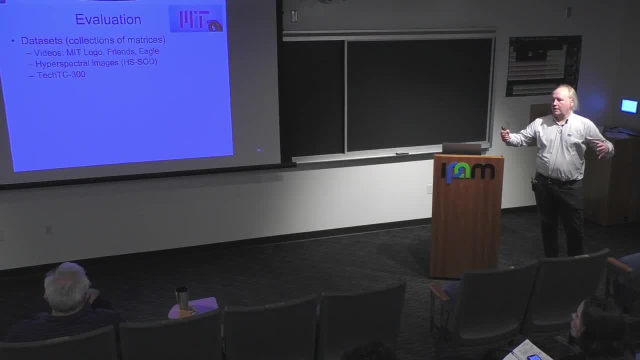 And it's important, you know This word. class is important, right, Because to train we have to have several matrices that kind of come from the same distribution, right? So so we cannot use many of the matrix data set repositories because they contain a single matrix, right? 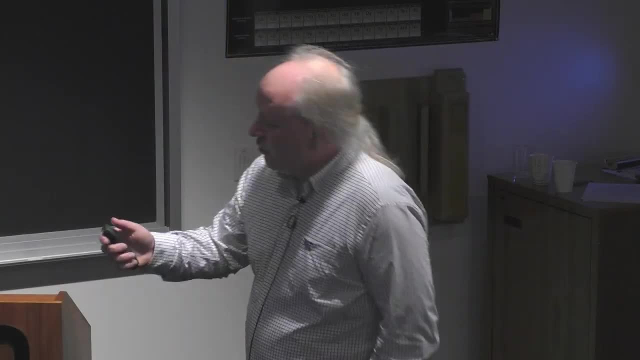 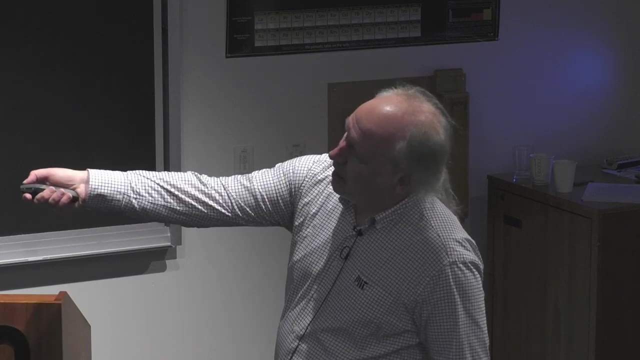 So, you know, we cannot really learn anything from that. So what we looked at is a, you know, collection of a data sets where indeed, you know you have a collection of us similar mattresses, One of their videos, right? So each frame is the matrix, right? 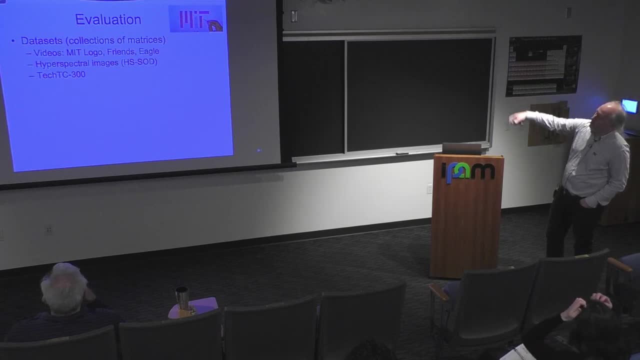 So we take any video, for example video of MIT logo being drawn or some other examples, and this gives you, you know, like frames are natural matrices which are of course, related. Hyperspectral images are another source, because you have matrices which are again related on different frequencies, and this is an example. 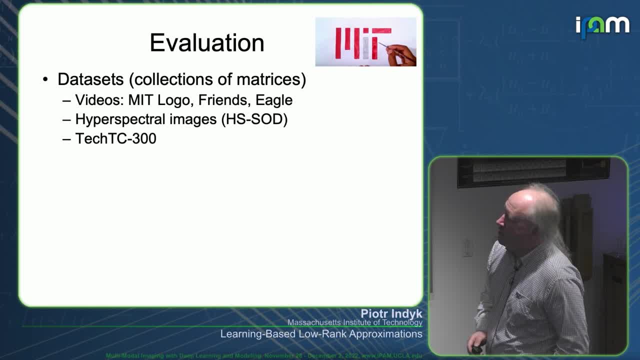 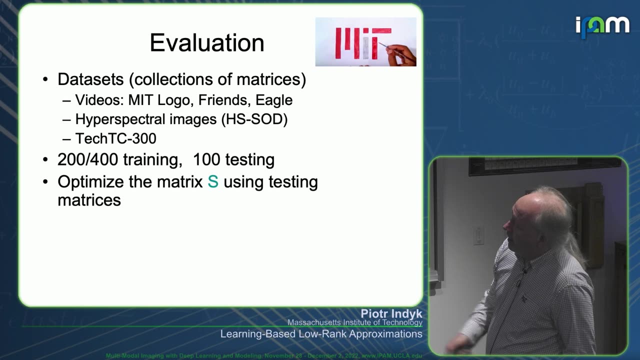 that I use as a matrix representation of documents, and these are documents coming from this similar source. We use a training set and a testing set to separate from training and we optimize the matrix S, as described earlier, using testing matrices and then we compute the recovery error over the test matrices. So this is the recovery error over. 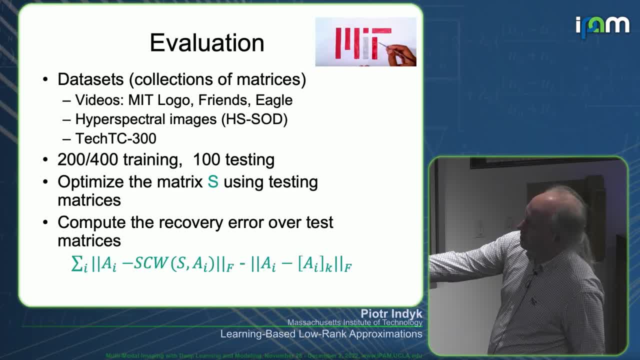 test is what we report on the next slide, and what we care about again is the difference between the error induced by the best case K component approximation and the error induced by the best case K component approximation And what our algorithm reports, right. so this is this extra error right that we are inducing by 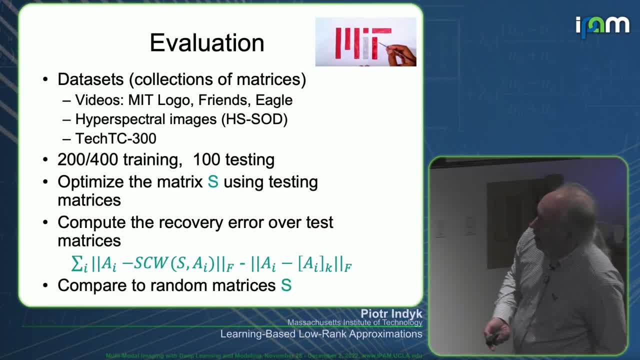 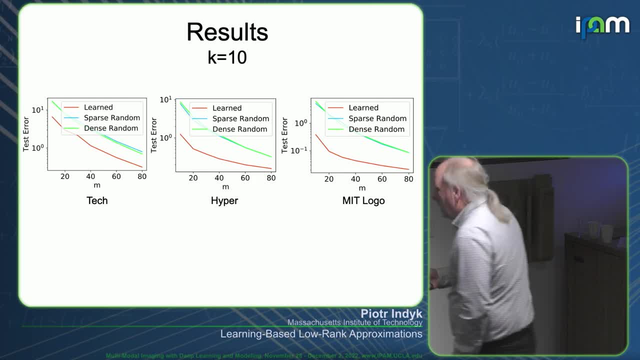 using this approximate algorithm And we compare this to what happens. we just use a random matrices, right as in the classical algorithm. So we did it and, to our pleasant surprise, it turns out that, at least for the data cells that we tried things on, you can indeed get a lot of mileage. 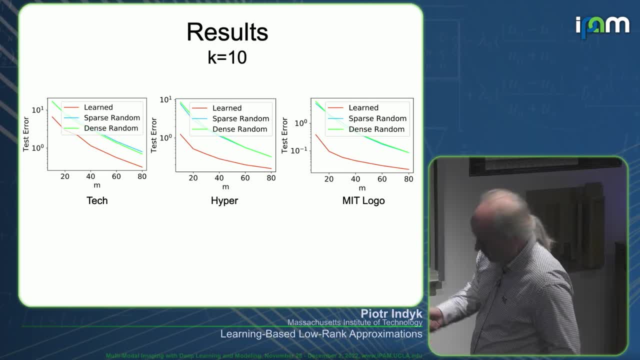 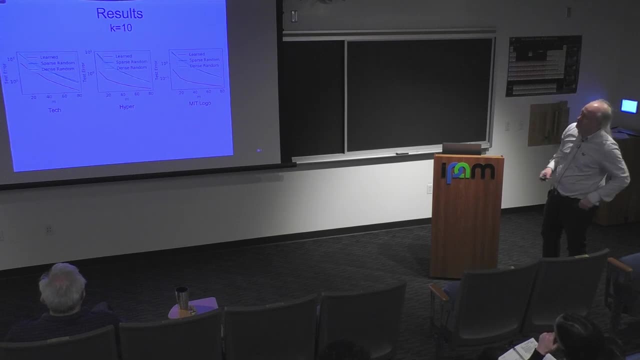 by optimizing those values of no zero, of no zero entries in the matrix S. So the plot that you see here is that test error right, as described in the earlier slide as a function of m right, which is the number of rows in the sketching matrix. So, of course, the more 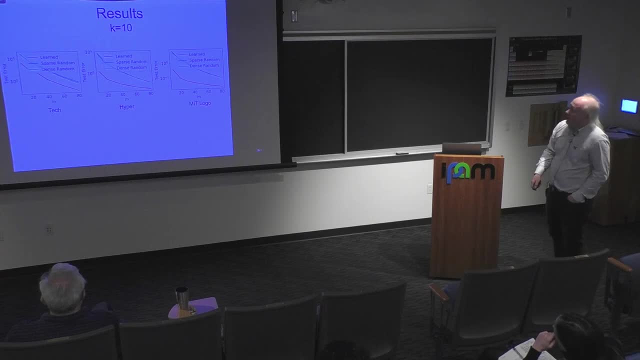 information you sketch, you know the, the lower the error is. You can see that there is a quite significant gap between the random matrices And the train matrices, right? and this is exponential, it's a logarithmic scale, right? so you know, here the difference is maybe not significant, here it's actually. 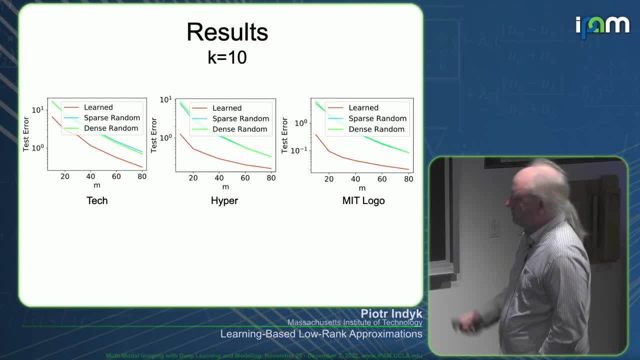 like, up to order of magnitude right and similarly here. So basically, what this shows is that, indeed, if you optimize, if you learn that matrix- as opposed to using random matrix, you can actually reduce the error for the same number of rows quite significantly. So this is perhaps the main finding of the paper. Now, of course, you know, as I mentioned earlier, you 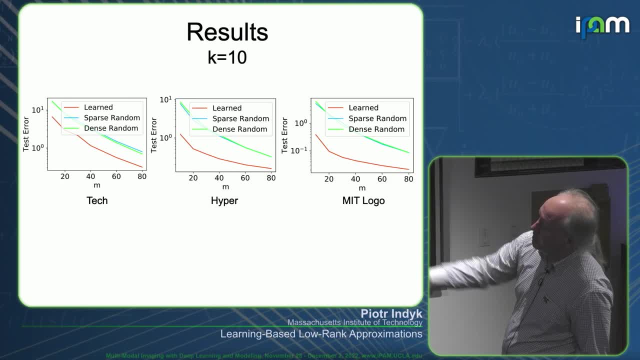 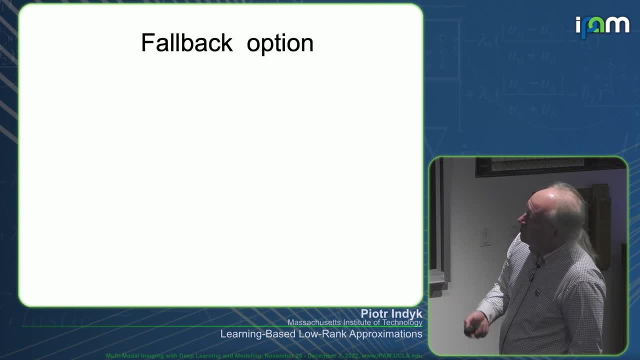 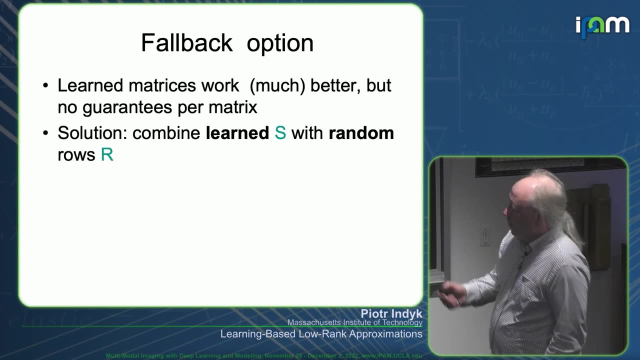 know, once you start using this optimized matrices, you lose guarantees, right, that you might have had earlier when you use random matrices. So what can you do? well, it turns out that, in in case of this algorithm, there is a very simple fallback option, which is that you can combine this learn matrix. 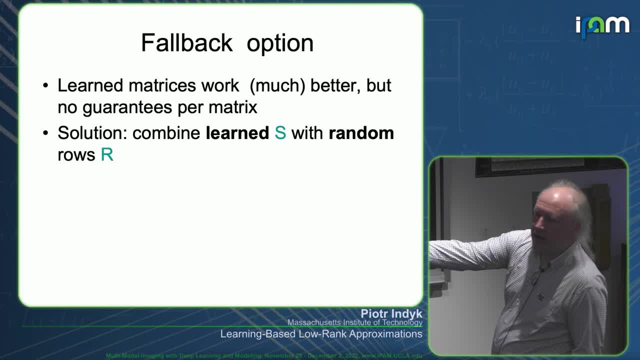 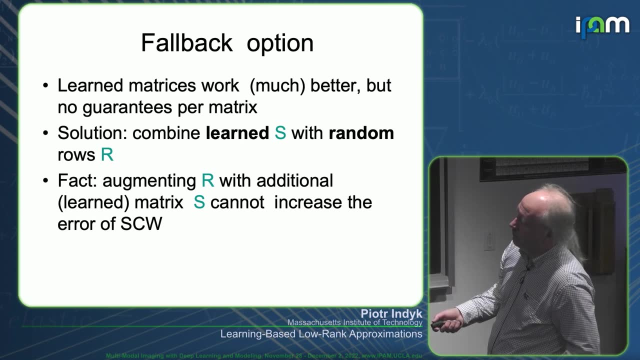 with some extra learning matrix. So what you can do is you can add some random rows. okay, you can literally stack them on top of each other. it doesn't work for all algorithms, but it does work for this scw algorithm. that requires you know like a few line proof. 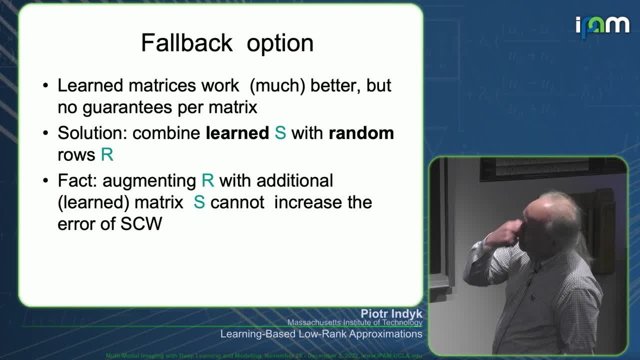 Essentially, what you can show is that adding this random r on top of matrix s cannot decrease the error And at the same time, you know, conversely, it means that adding this s on top of r also cannot decrease the error right, which means that we retain the guarantees, whatever guarantees this matrix r here gives us, while 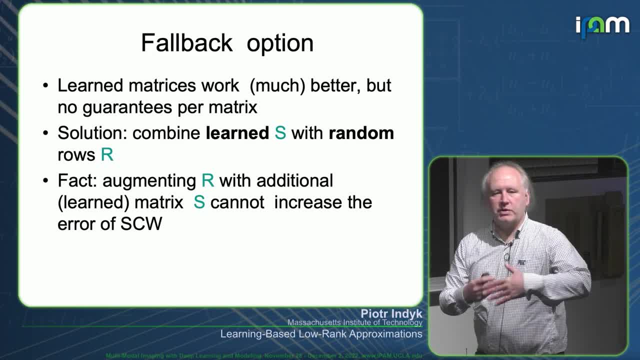 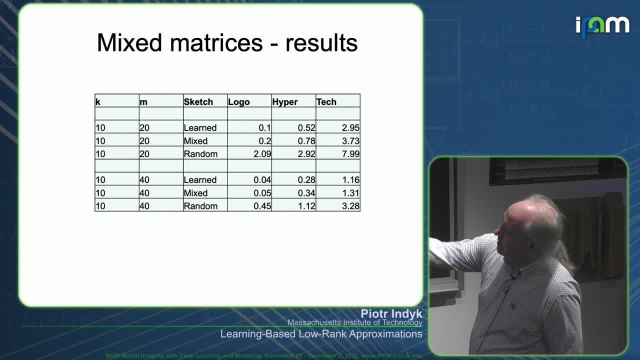 potentially improving things by a lot, because we are also using this learn component. okay, So here is an example of how it works. okay, so you know, for different data sets, you know, and different parameters of KNN, You know. here are the empirical errors of the purely learned matrix. 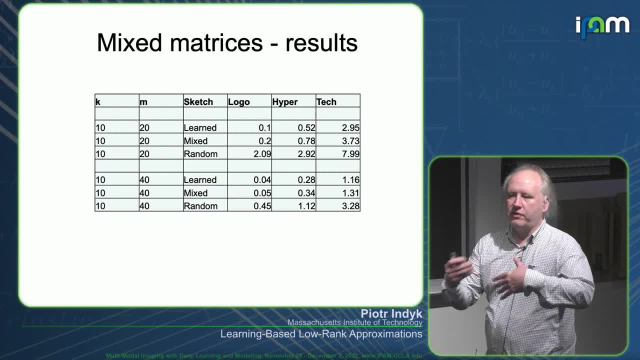 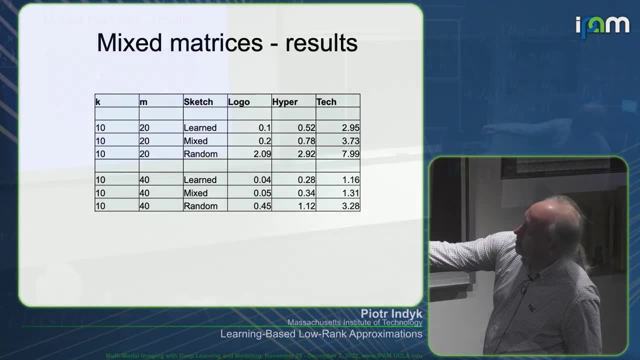 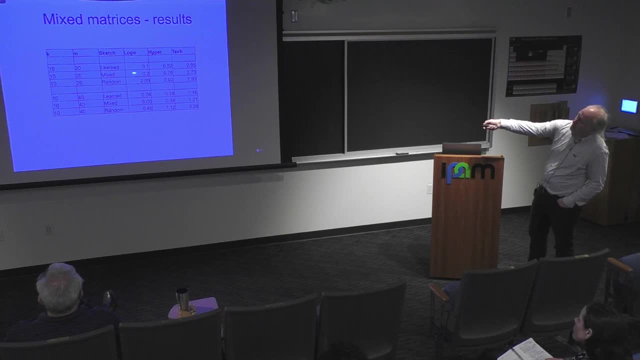 purely random matrix and the mixed mix means it's like 50, 50, right. so it's: the total matrix still has the same length, the height, 20, but here we, one half of it is learned, the other half is random, right, and you can see that. you know, of course mixed doesn't give you the same empirical error. 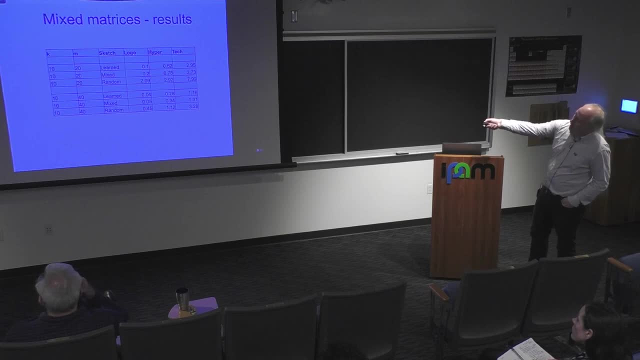 as purely learned. right because you are learning fewer errors, but still it's pretty good. right. Most of the times it's actually closer to the learn than to random and at the same time you retain the guarantees whatever this random component gives you. right because you can. 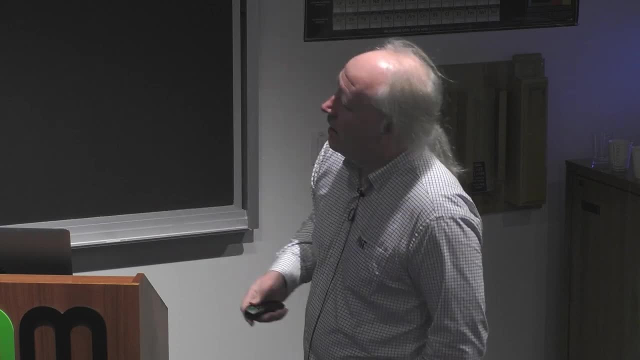 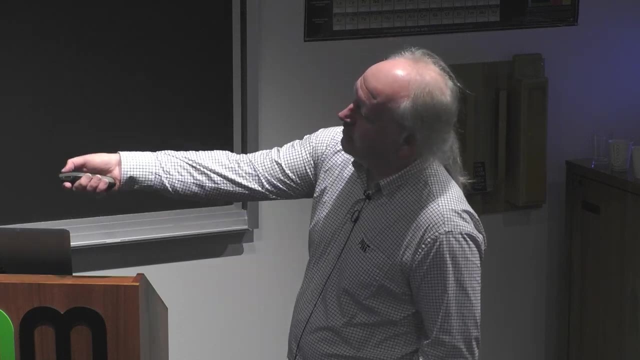 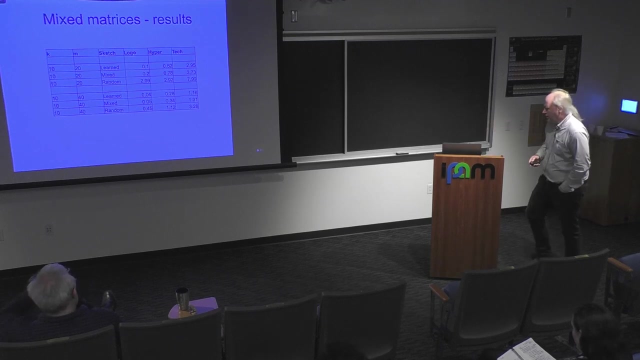 just directly translate it into guarantees of this algorithm, right? so in a way, you know this could be viewed as the best of both worlds scenario, right, that you are learning and you know you are doing better, but you also retain some guarantees. Question: Yes, In the mixed case, do you learn the features with those random? 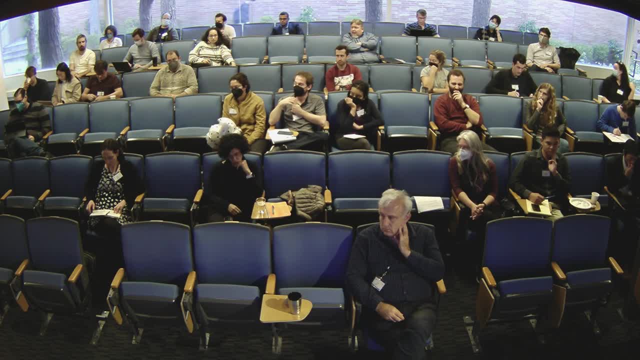 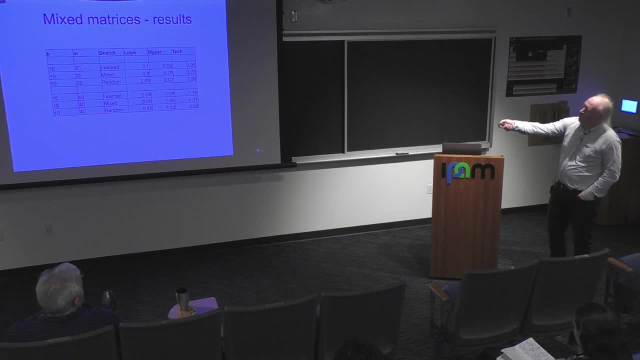 settings or do you first learn the first 10 and then just concatenate random? I guess, if they learn condition to the randomness of the second half, Right? so if I remember correctly, we learned jointly with the random component. is just that component is not modified in the learning process? yeah, I think what I said is true. it was like 90. 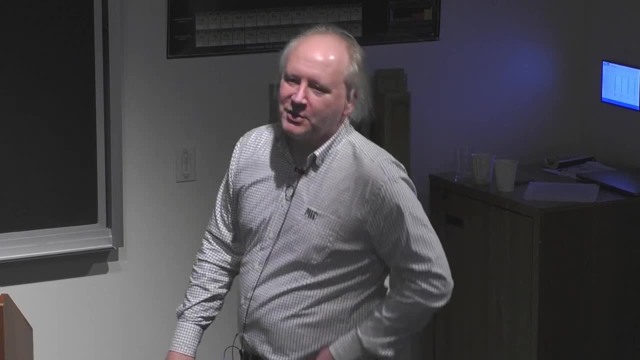 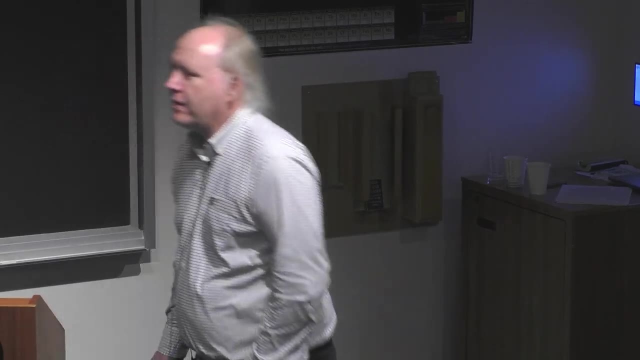 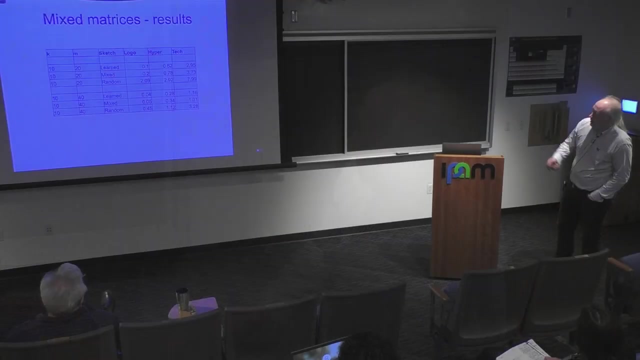 percent probability. I will have to double check too, All right. so let's see, I have like 10 or 15 15 minutes left. 15, 15, all right, okay, all right. so. so that's basically was something that we did in 2019.. 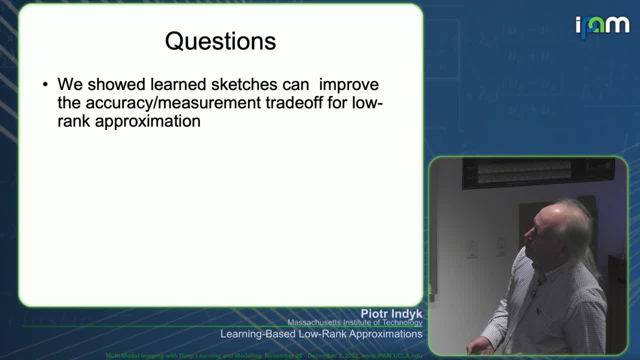 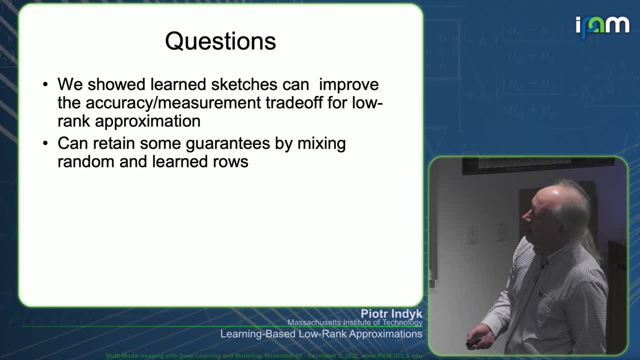 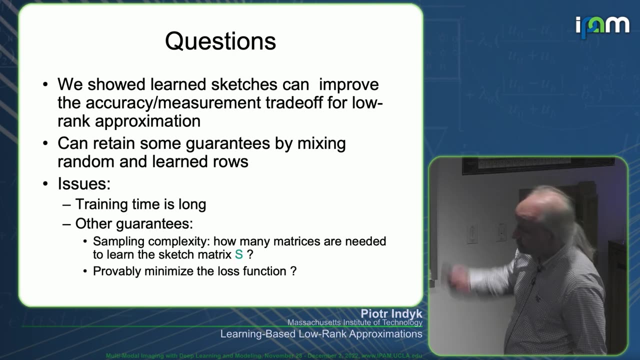 In particular, you know, like the bottom lines, that we showed, the sketches can indeed improve the accuracy measurement, And we also showed that you can retain some guarantees by, you know, mixing random and learn rows right. so so that's nice. Now, that said, you know this algorithm still has lots of issues. 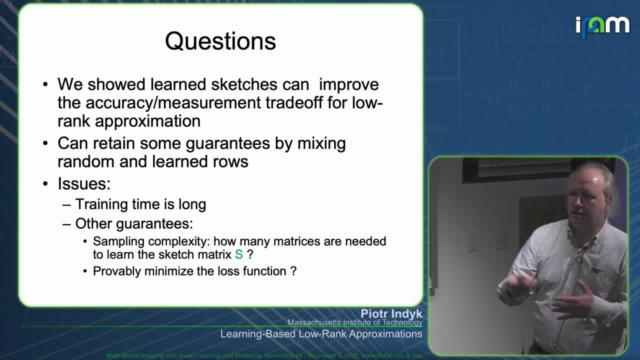 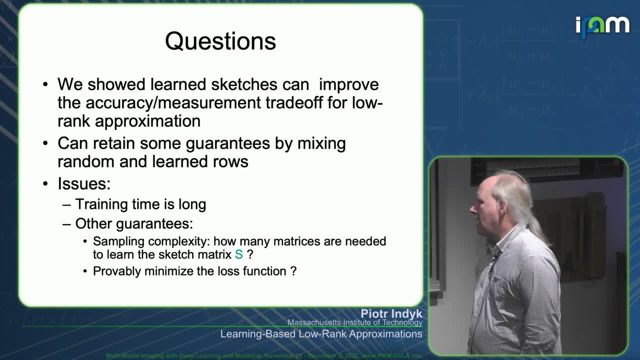 One issue is that the training time, which is, you know, optimizing this non-convex objective function, is really long. right, it took us hours on github And it also takes a lot of time to make sure that we can use this matrix, or you know the. 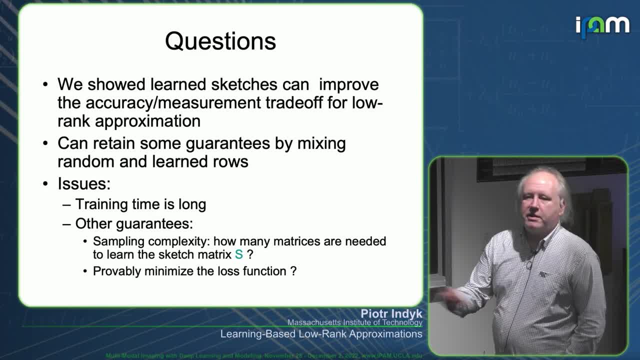 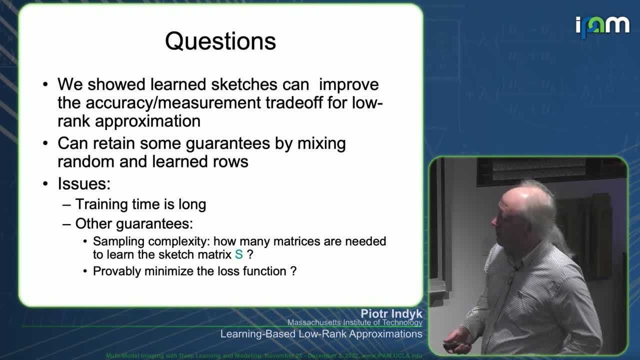 the gpu to train this matrix, which you know. it's probably okay. if you are going to use this matrix for the next year, right, but if you want to use it for the next- like every five minutes you know we want to change it- then then just not gonna fly right. so that's one issue. the other issues are: 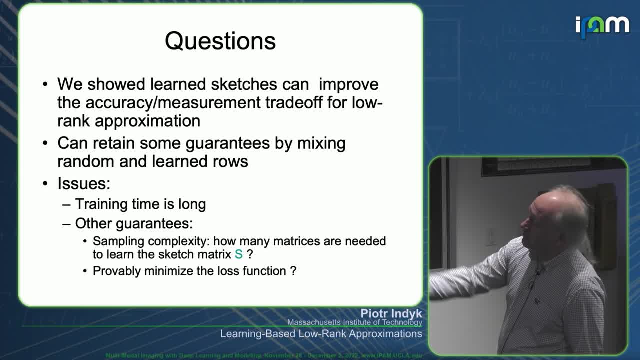 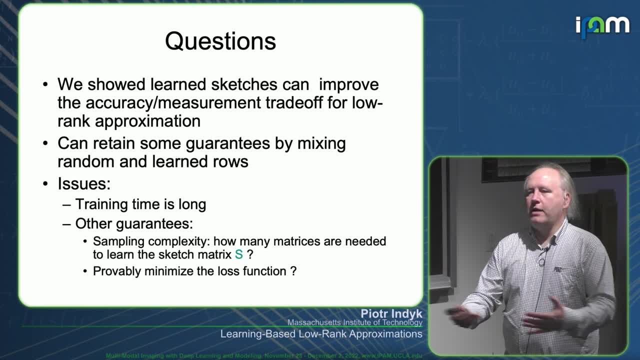 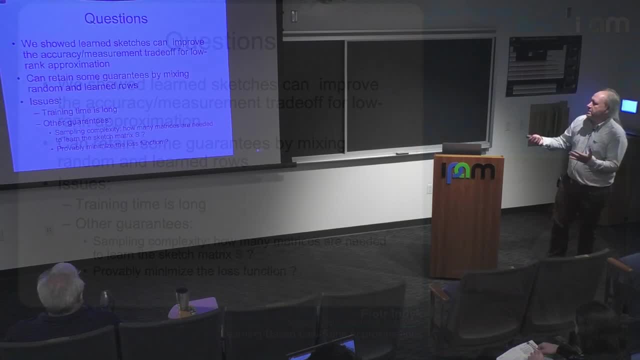 more theoretical, which is: it would be nice to have some guarantees that if we, if our data set is large enough, we actually, in principle, find this optimal matrix S up to some error. right, Like right now, we just have no clue. right, We're just putting as many matrices as our data set has and hope for the best. 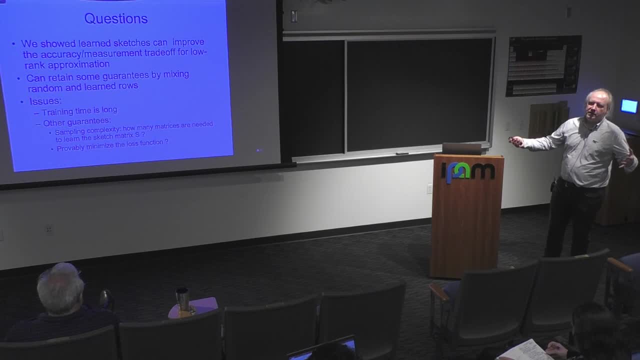 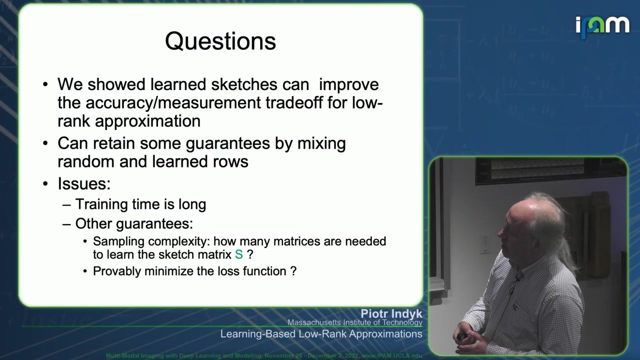 but we have no theoretical guarantees Like how many matrices we actually need right to get the optimal sketch matrix S. So that's one question or another question. And you know, and last but not least you know, we are using stochastic gradient descent to minimize this function right. 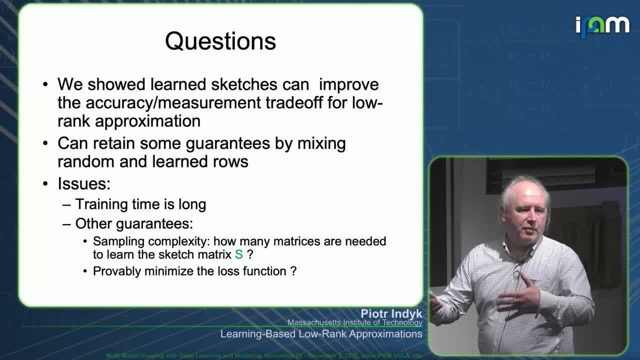 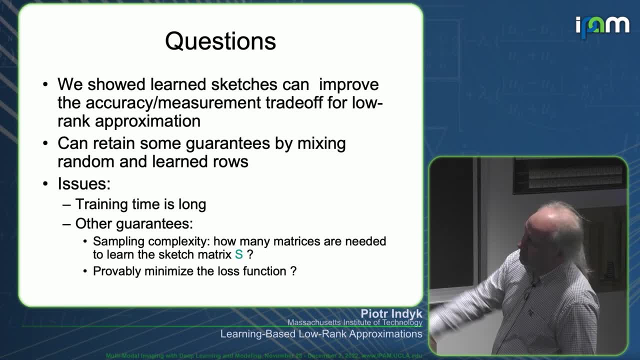 We are stuck at local minimum. We have no idea how far this local minimum is from the global minimum, right? So getting some algorithm which probably minimizes loss function up to a constant factor would be super interesting, right? Especially if it can avoid, you know, this gradient, descent, you know. 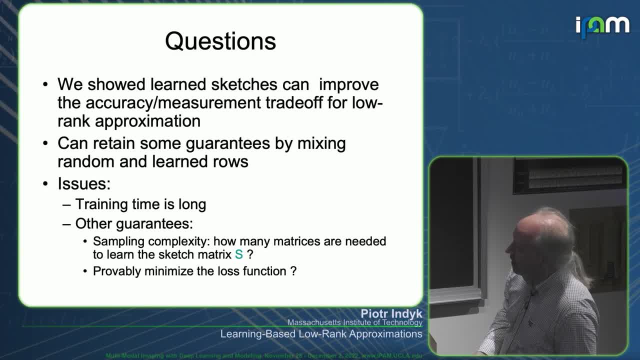 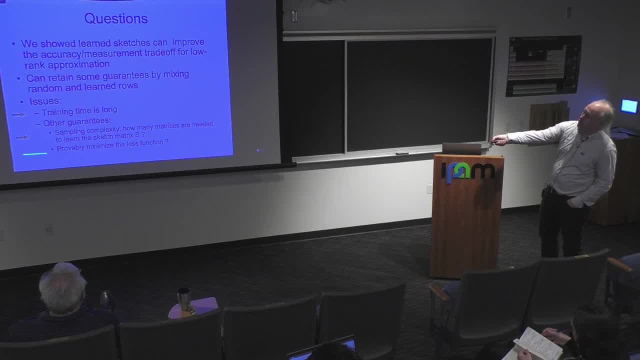 if maybe there's some more direct way of doing it. So these are the problems that we are thinking over the last three years. We still don't have an answer to this one, but we do have some progress on the training time and on the sampling complexity. okay, 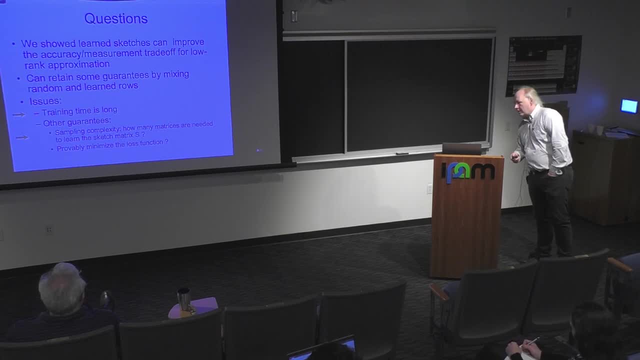 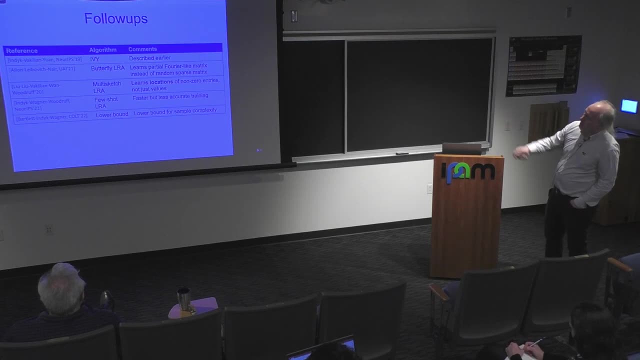 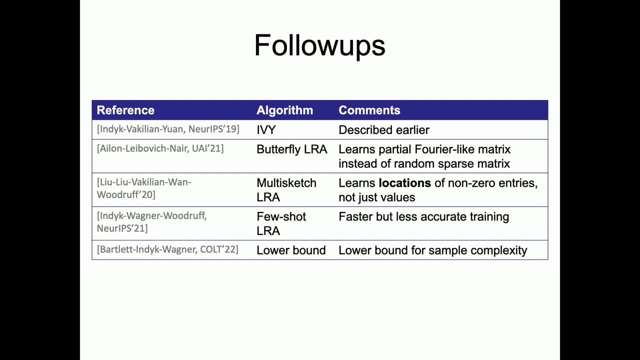 So this is what I will briefly cover in the next 10 minutes or so. All right, so after our work in 2019, there have been a few very, very cool follow-ups. Most of these follow-ups focus on a different training method. 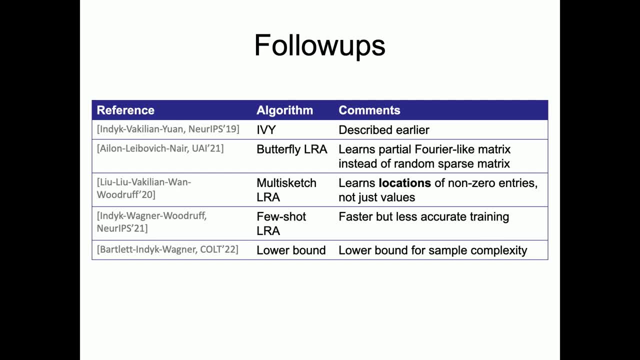 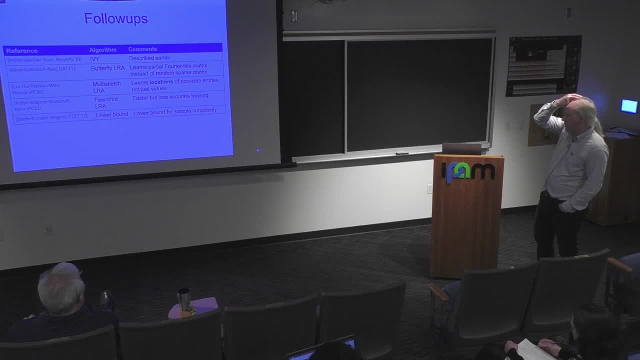 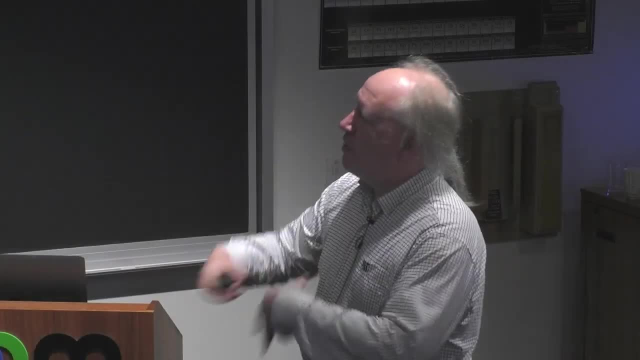 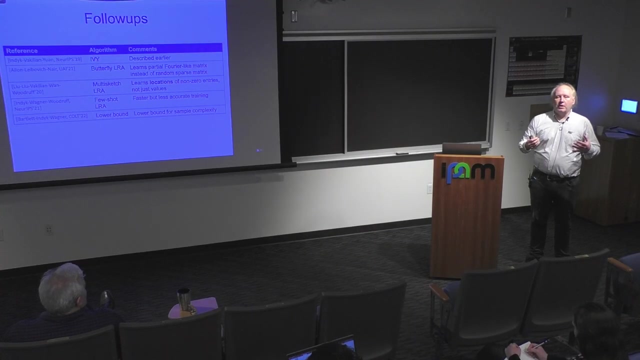 or training different type of matrices. okay, In particular, this work is very interesting. Essentially, you know, in our case we learned random sparse matrix or we optimized over random sparse matrix This paper tracks. This paper tracks random partial Fourier-like matrix, right, 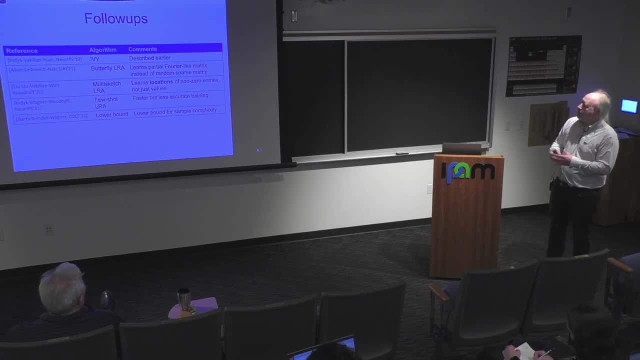 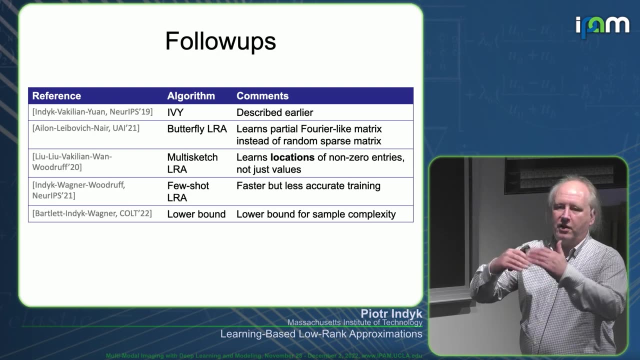 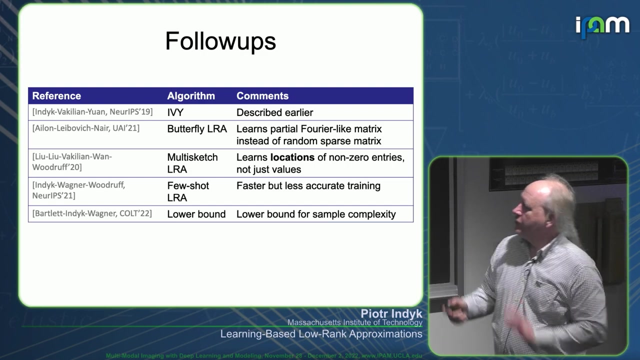 So what it means, you know. Fourier matrices are basically a product of sparse matrices, right? So with a, you know particular value, with particular values, right, You know the roots of unity and so on. So this algorithm retains the structure of those matrices but again learns the values, right? 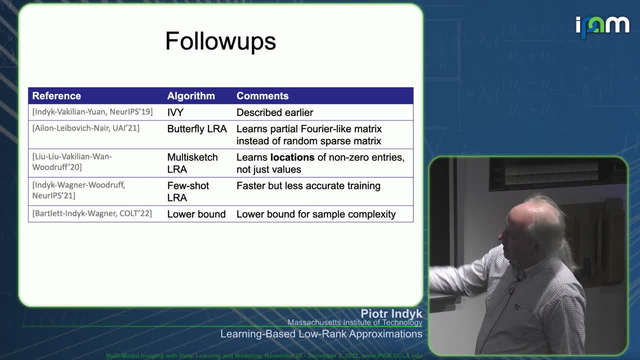 Instead of just keeping them fixed. So I'll show you on the next slide. you know it's. you know, because of this different type of a sketching matrix, that this method learns. you know they are getting, in a variety of ways, much better algorithmically. 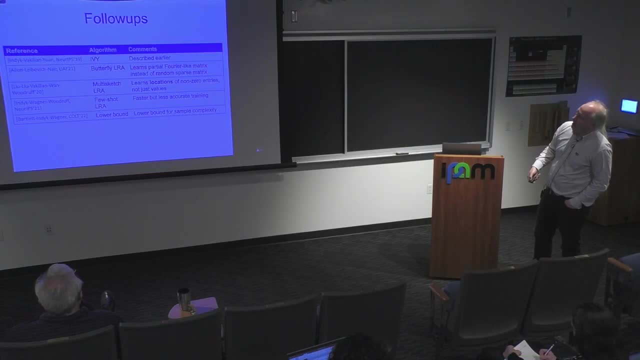 And there has been also work on learning locations And we had a paper last year which shows a faster algorithm which doesn't go through all this stochastic gradient descent. It's more. It's more like a one-shot or a few-shot learning. you know that you sample a few things. 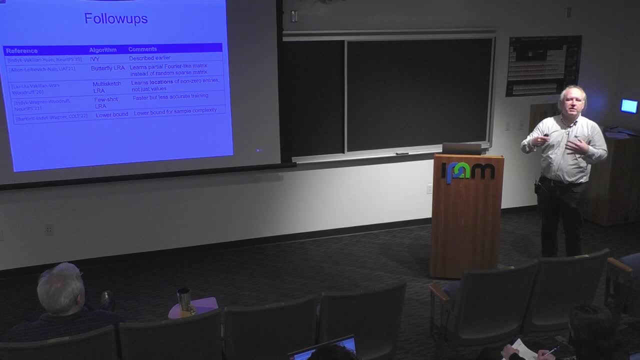 and based on those few matrices that you sample, you construct the sketching matrix right. So it's not as good as this one, but it's much faster. So these methods here improve essentially the training time. This method, this paper here which just came out this year, 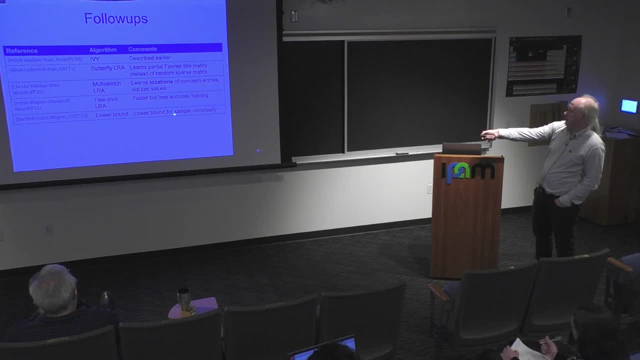 for the first time, shows lower Oops- actually it should be both upper and lower bound On the sampling complexity of this problem right- So we're able, for the first time, to show how many matrices you need in order to get some guarantees right that you are close to the optimal sketching matrix. 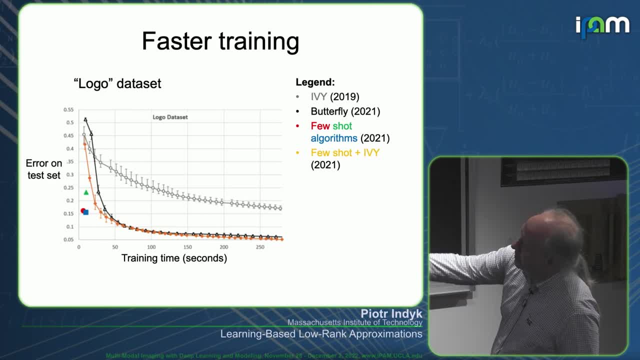 All right. So let me briefly summarize the work on improving the training time. So what you see here is an example of this training process on a logo dataset. So this is one of those videos, So data sets. This is an improvement, like as a function of time of the error in our method from 2019.. 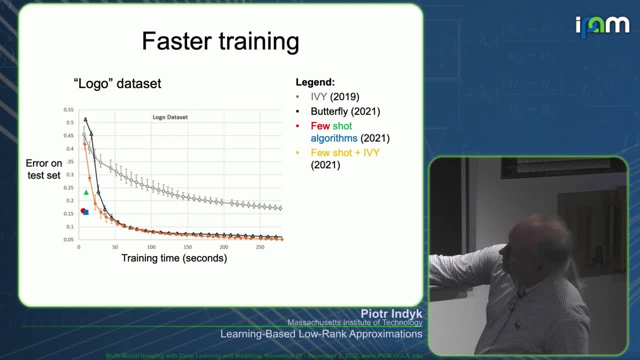 The butterfly method right, which I just described on the previous slide, is this black curve, And you can see that it's way, way faster than It converges or, you know, achieves a near optimal, much faster than the previous method right. 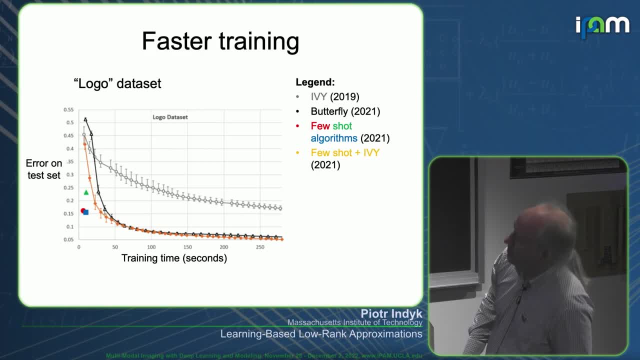 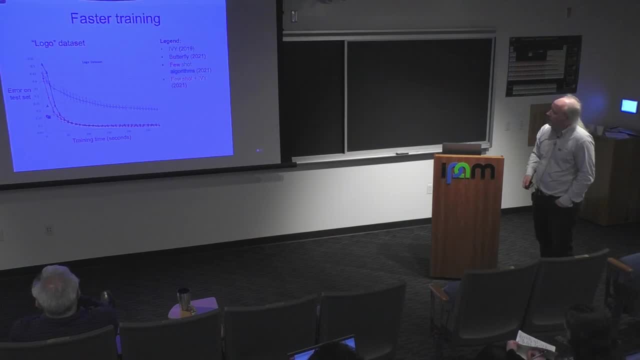 I mean this method. you know this is not the optimum, It just continues, but very slowly, right, Because it reaches the optimum. This method jumps to optimum much faster, And we also had the few-shot method that I mentioned earlier. 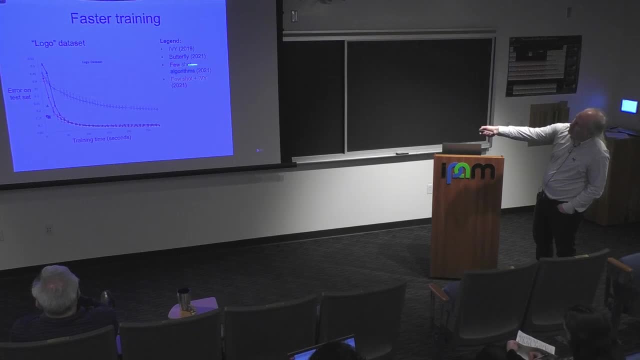 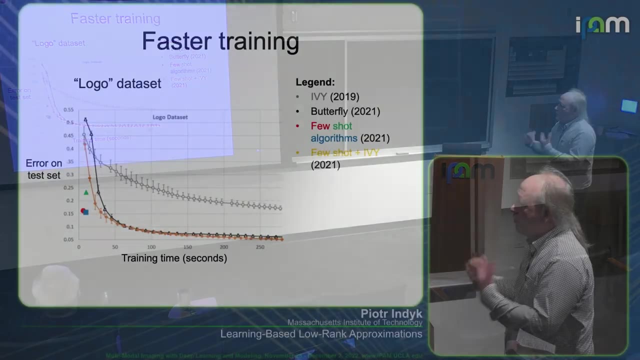 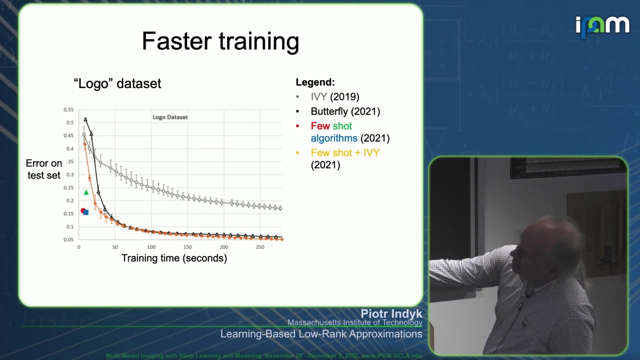 It's not as good as the optimum right. The few-shot are depicted as red, green and blue dots here. okay, They don't improve over time, But they are fast, very fast at starting points, right. So what you can do is you can take those as initialization. 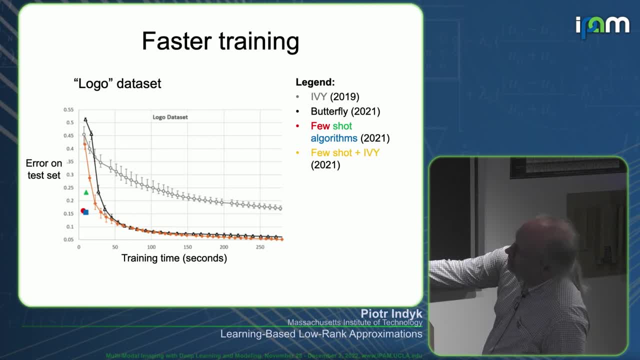 and then you know, run a gradient descent on them and then you get also very efficient, very fast improvement. okay, So this is, you know, just an example showing that you know, thanks to these new methods, you can actually train this thing much faster. 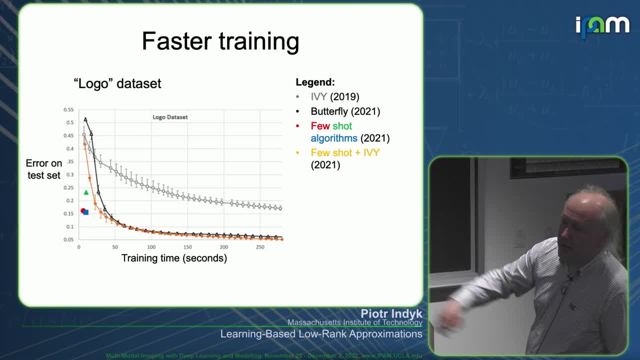 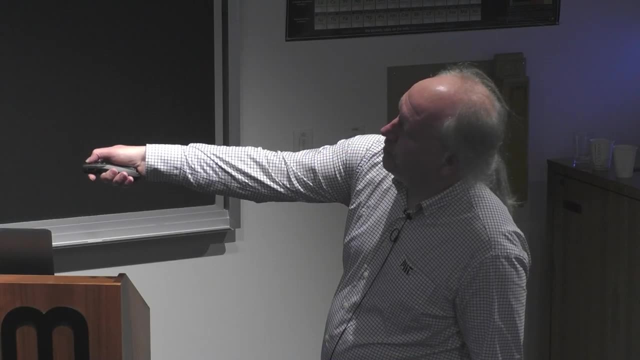 I would say that part of it is just a better implementation of the training process in Python, right, Like, to some extent, we weren't quite, We didn't quite know what we were doing when we wrote this paper, right. So it's both a better implementation, but it's also, you know, 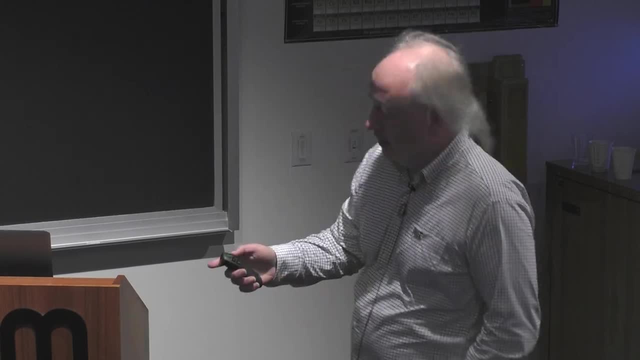 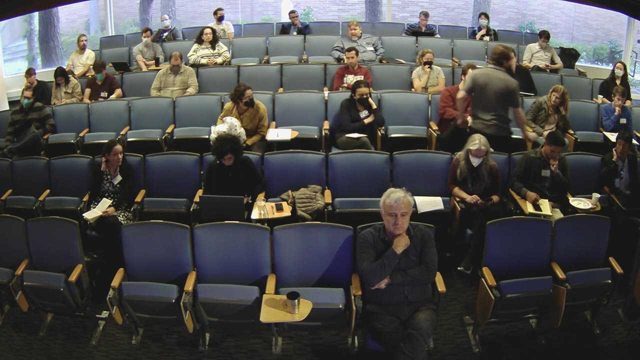 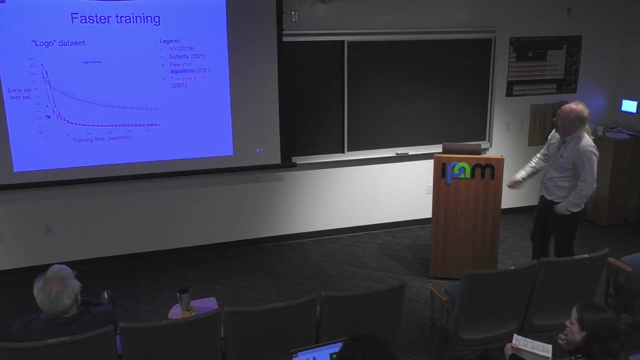 like using different algorithms and different matrices. Yes, For the training. so are you using GPU or just using this? Okay, so this particular- Okay, I believe this plot is done on GPU. Yeah, Just one GPU code On a machine with multiple GPUs. 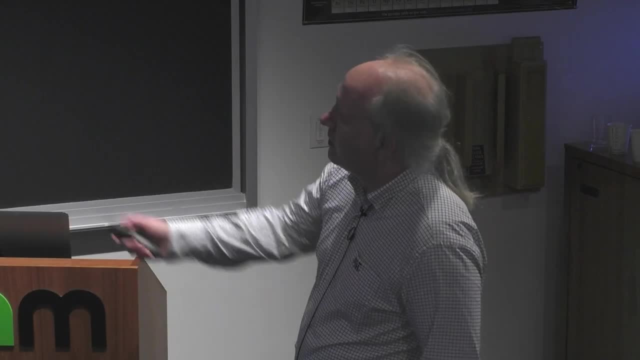 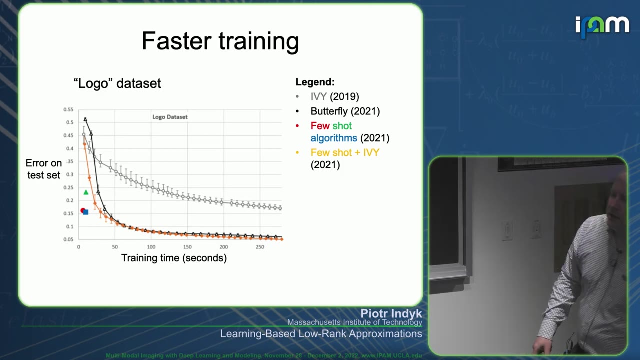 Yeah, I don't remember exactly the architecture It should be. This plot is taken from this paper, right? So in that paper we described the Yeah, that's Yeah. Yeah, this method was very slow without GPUs, so 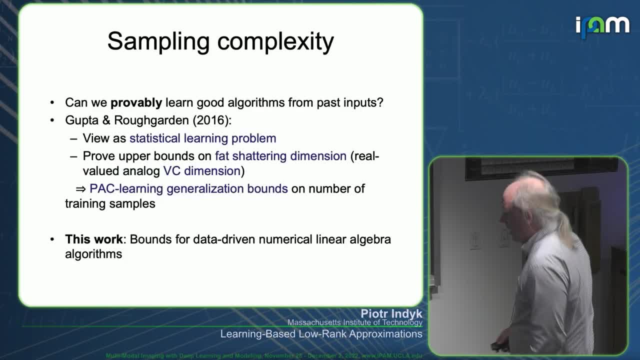 All right. So that's the faster training. Now, in terms of What about the sampling complexity right, Trying to get the You know some bounds, How many matrices are necessary and sufficient to You know to find near optimal sketch matrices? 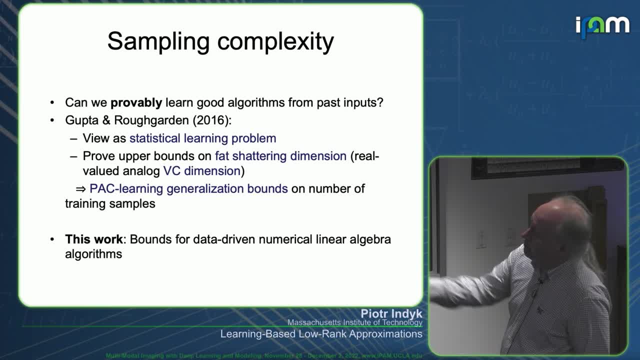 So to this end, we use a framework due to Gupta and Aerofgarden, Who essentially view this problem of learning algorithms as a statistical learning problem. right And essentially, once you put your problem in this framework then you know it's a statistical learning problem. 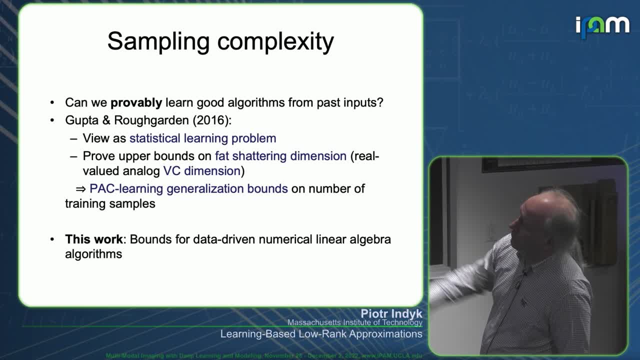 So you, You know it suffices to prove bounds on, you know BC dimension or some like real analogs, like fat shattering dimension of you know this class of algorithms, And it gives you basically statistical guarantees. 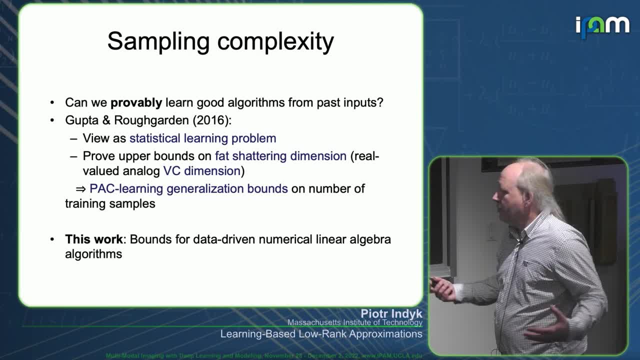 Right That you need that many samples or that many samples are sufficient to find near optimal matrix S. So in this paper we are applying this framework to you know, basically the numerical linear algebra algorithms for low-rank approximation as I described earlier. 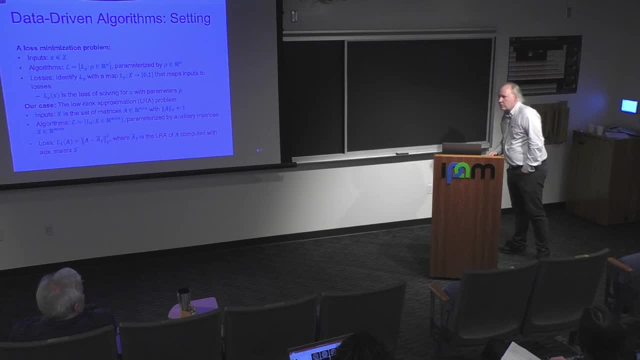 Now I don't think I will be able to. I have like five minutes left right But I don't think I will be able to describe this whole, This whole framework. But let me just give maybe a snapshot. 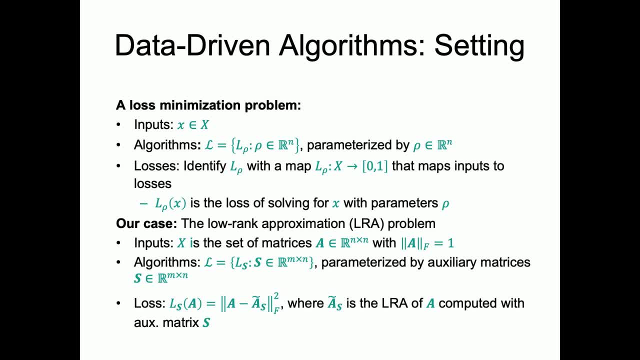 So the basic idea, you know, is to view this algorithm as a loss minimization problem, Right, So the inputs, you know, come from some family X And the algorithms are basically, you know, these algorithms are denoted by L, sub-heel-th row. 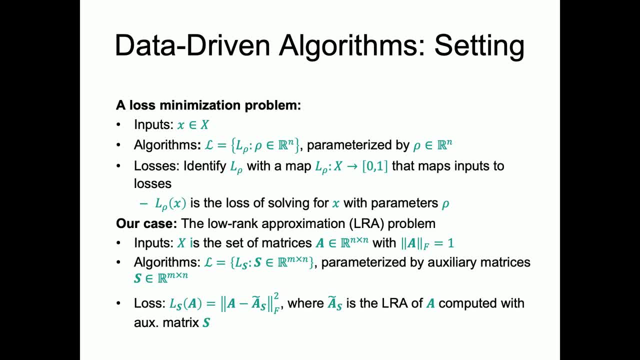 And this row is the parameter of this algorithm, Right, And Basically we think We think about this algorithm as a loss, Right, That if we run algorithm on a particular input then we have this much error, Right, And then our goal is to, you know, optimize the sub-parameter row with respect to some distribution. 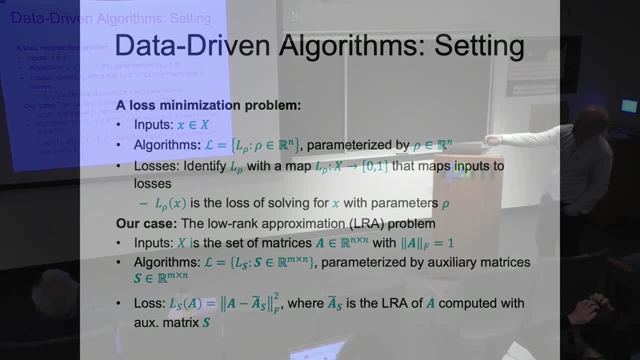 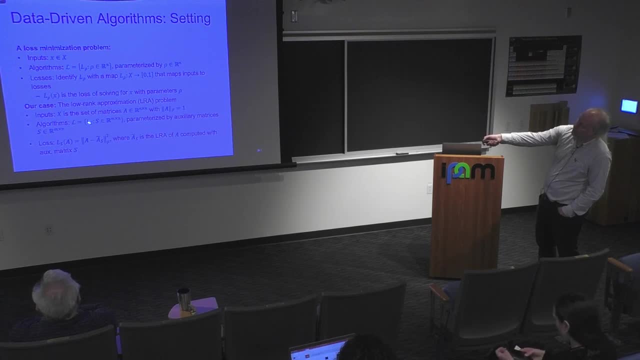 Right Over this input: X. Yeah, So in our case, you know, X is the set of matrices L, you know, are the losses incurred by the algorithm which use matrix Sketching, matrix S as a parameter, Right. 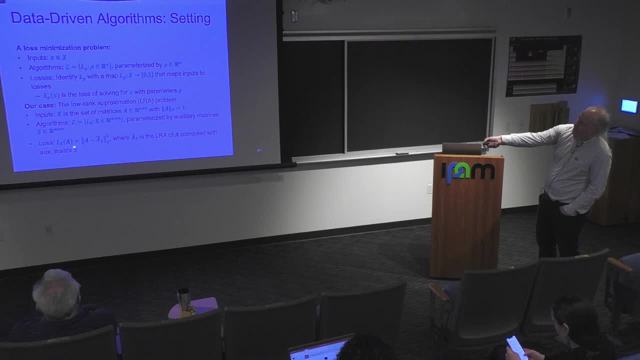 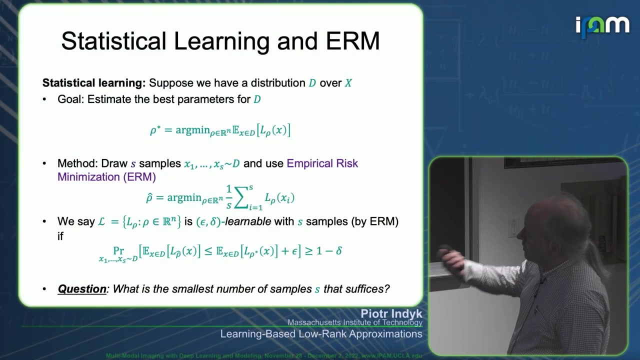 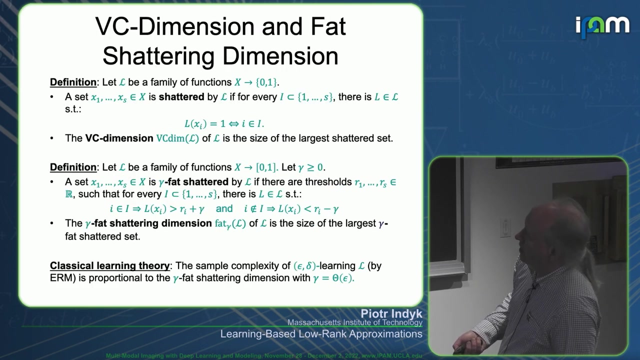 And This is our loss. Right, It's the difference between the truth and the Whatever our algorithm reports. Right, When applied on matrix A using sketching matrix S. And then there is, you know, And now we can just apply it in standard learning theory framework. 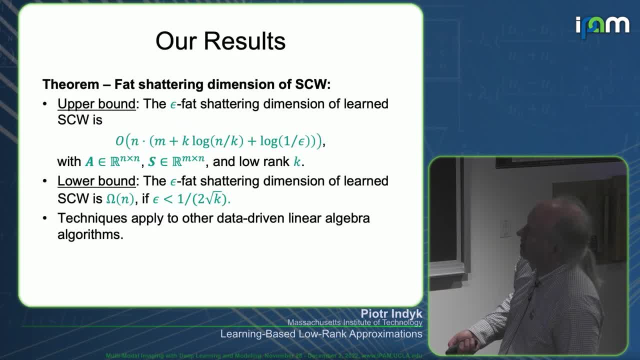 Right, You can start computing things like VC dimension, fat-sheddering dimension, So I'm going to skip all of it, But just let me state our final result. So, basically, we give both upper and lower bound on the so-called fat-sheddering dimension of this learning process. 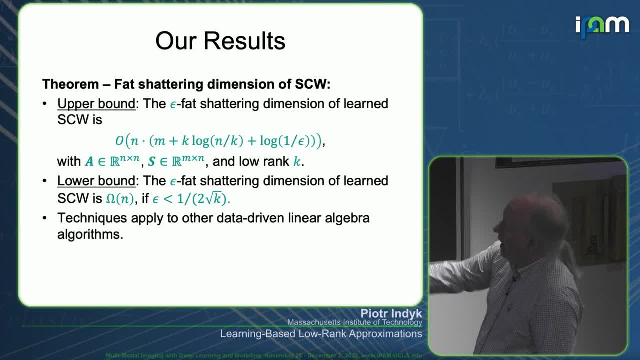 Right. And we have the upper bound, We have the lower bound, And you can see that the upper bound and the lower bound differ by essentially a factor of N Right. So they are not optimal. At least we don't know which one is the optimal. 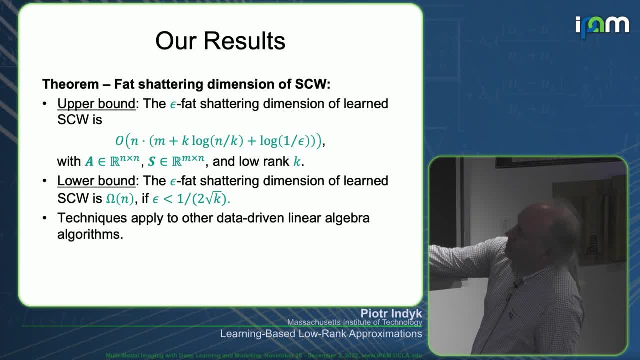 Right, They are not tied, But they are actually pretty close, Right? So we have at least some sense of what this learning parameter of this process is, And once we have this fat-sheddering dimension, we can then plug it into classic complexity theory results. 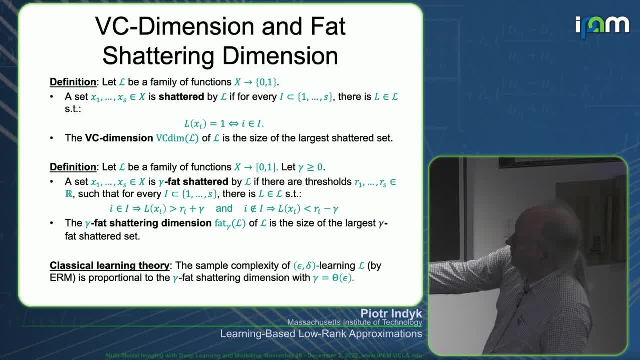 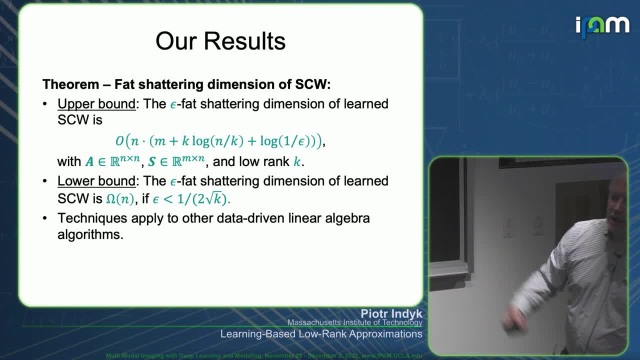 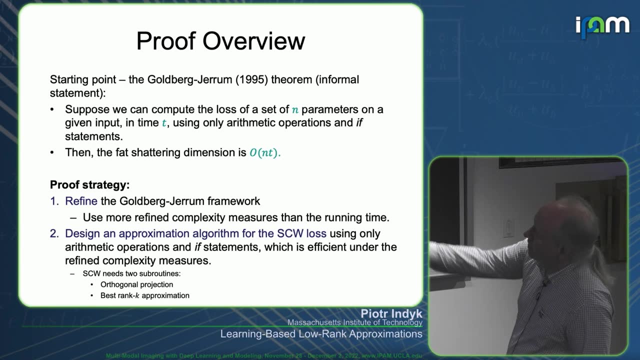 You know, which basically shows that the number of samples is proportional to the fat-sheddering dimension, Right? So by plugging this bound Right, We get the bounds on the sampling complexity of the process. I won't have time to get into how we do it. 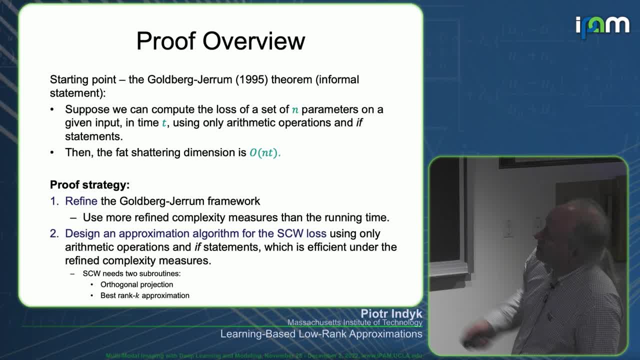 I just mentioned that. you know, we're stuck on trying to get those guarantees for a few years Until Peter Bartlett, who is the co-author of this paper, mentioned to us the similar paper by Goldberg and Jerome, Who essentially came up with a very general framework for computing. you know, 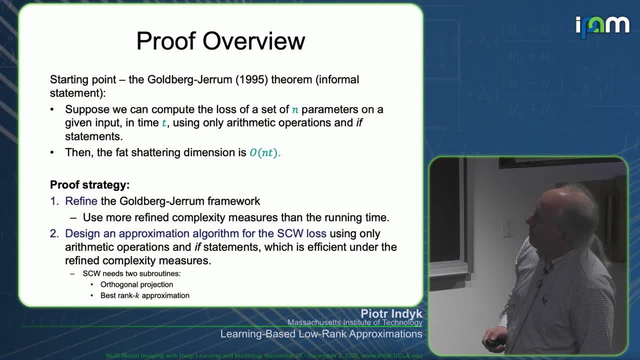 which is called the linear algebraic dimensions, or a fat-sheddering dimensions of programs which use only arithmetic and if statements. Okay, So this framework was pretty crucial to obtain what we wanted to do because, you know, linear algebraic computations exactly fall into this setting. 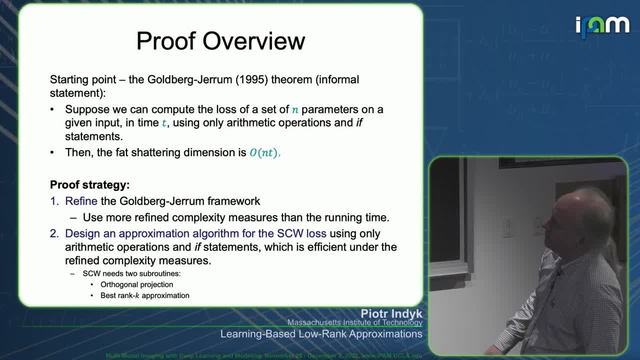 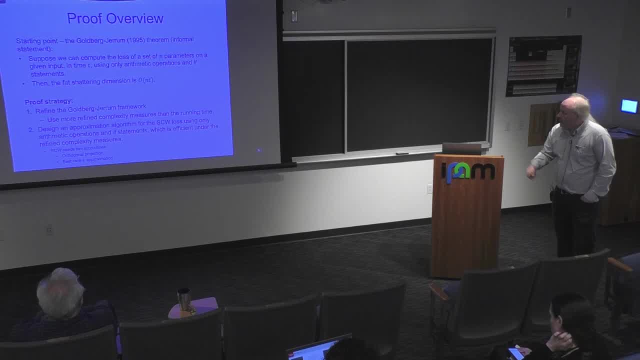 Right, You only use arithmetic operation. You have some if statements here and there. We tried to use a combinatorial approach and it just didn't work Until we found this paper. Now, if you apply this method naively, you are not going to get very good bounds. 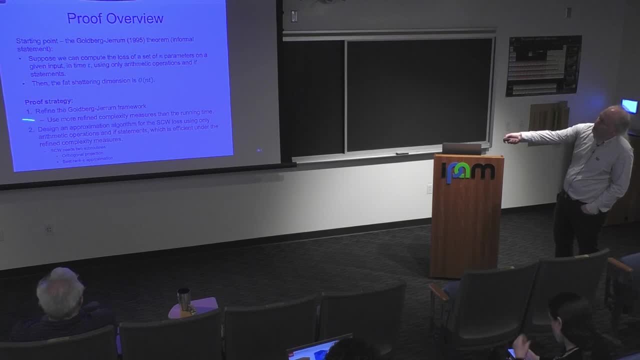 So, basically, we look a little bit more. you know, we don't treat it as a black box, We treat it as a white box, Right, We try to refine the complexity measures that they are using And then we essentially design approximation. 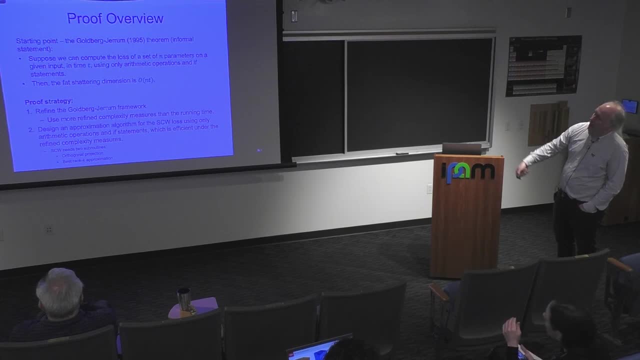 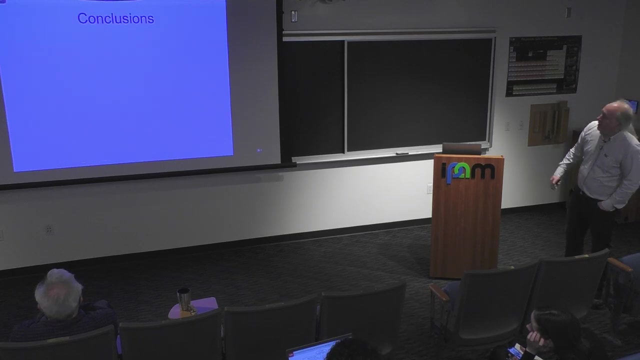 We implement the SCW within this framework. You know, essentially we implement the start-to-end projection best-ranking approximation in this framework, which then lets us to get this not tight but reasonably close upper and lower points. All right, So that's in conclusion. 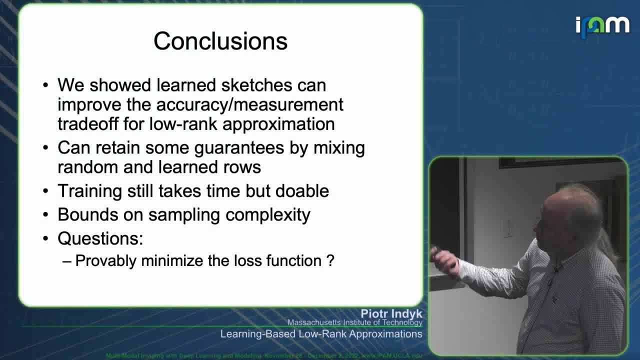 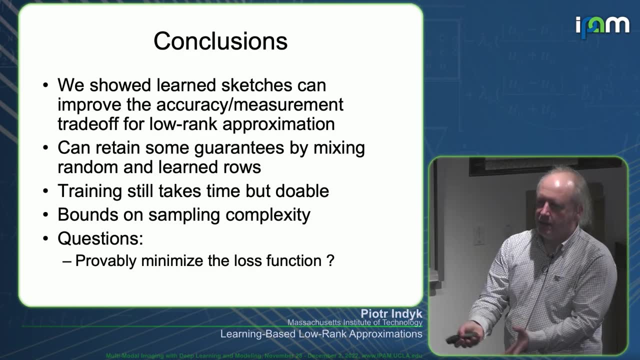 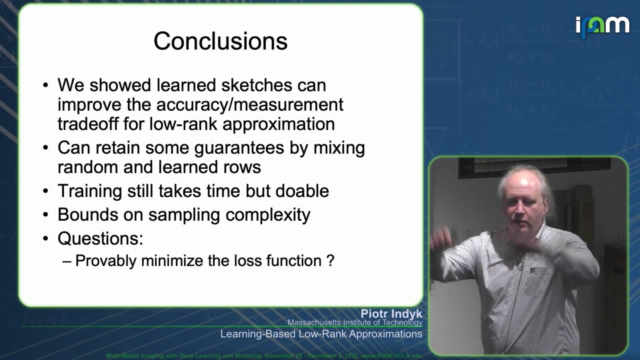 Right. What we have seen is this. Perhaps the main open problem is: can we somehow minimize the loss function? Probably Right. So that could mean two things: Either giving guarantees on this SGD, on this gradient descent, or maybe come up with some more direct way to find this matrix S right. 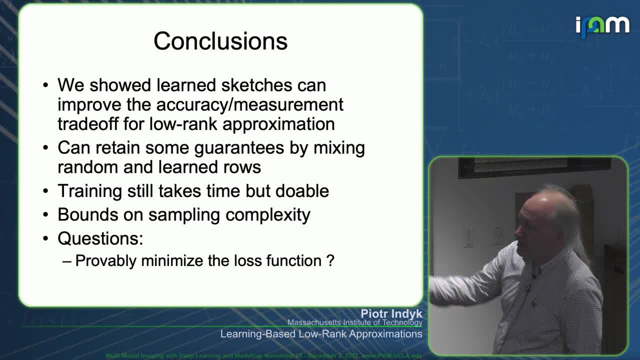 Without going through all this minimization Right. So that would be, you know, having any insight here would be very, very interesting And this potentially could, you know, improve the training time even more Right? Especially if you don't have to go through gradient descent right. 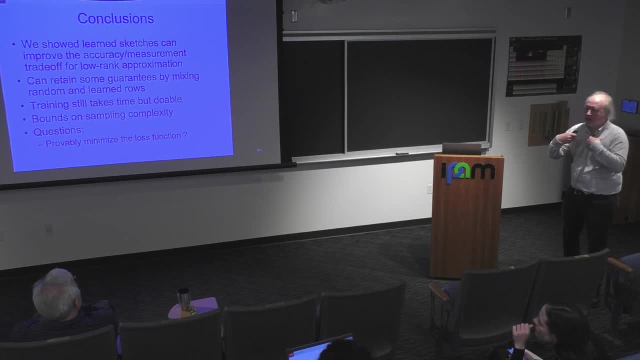 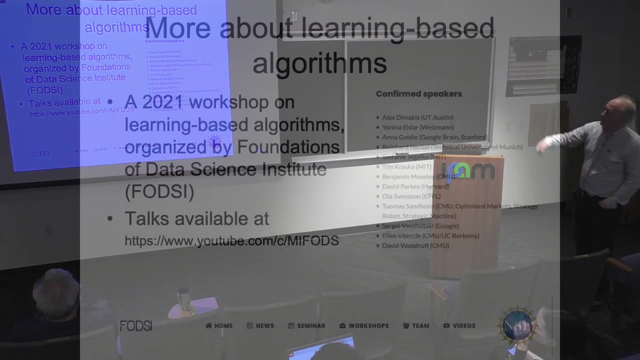 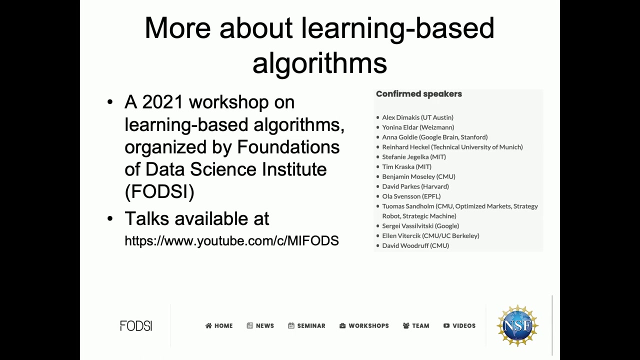 You have some, you know, explicit formula Right That just calculates as a good sketching matrix based on the input matrices. And, last but not least, this is, you know, like a one line of research in a broader area of so-called learning-based algorithms. 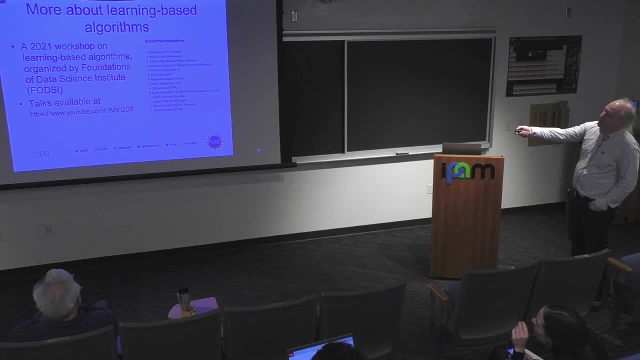 And most of the algorithms in this space are combinatorial, but you know like some of them are also numerical, Right. So, in particular, I talked about one of the example right. so a year ago we had a workshop organized by foundation of data science Institute. 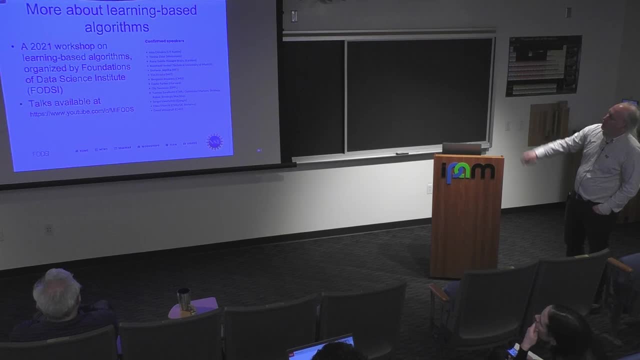 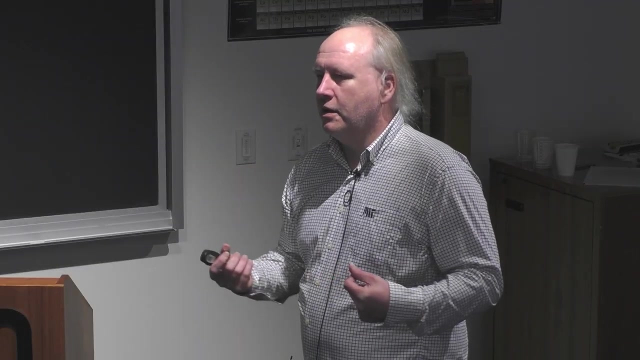 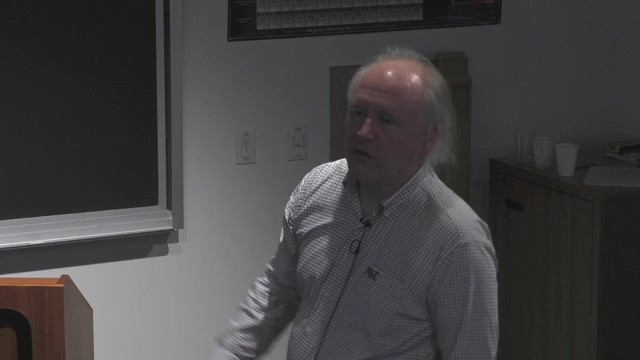 with speakers you know gave a broad overview of research in this area. and for Alex the Marquis, you, Nina Eldar and the Ryan Ryan Reinhardt, Reinhardt, right, talked about learning augmented numerical algorithm, right so? so if you are interested in learning more, you know the talks are available here, right so?